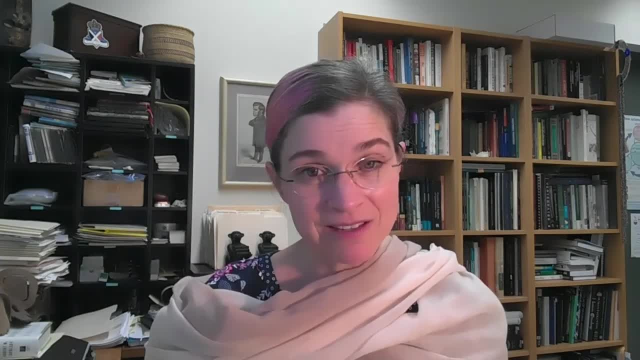 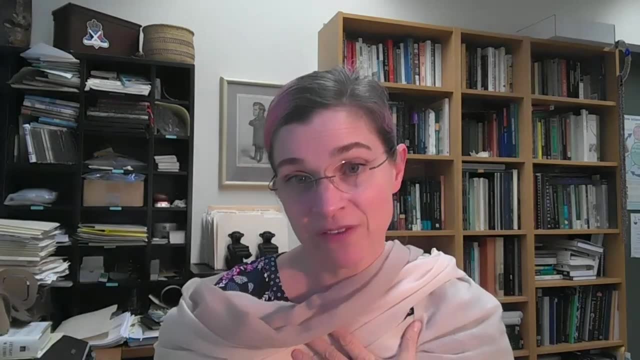 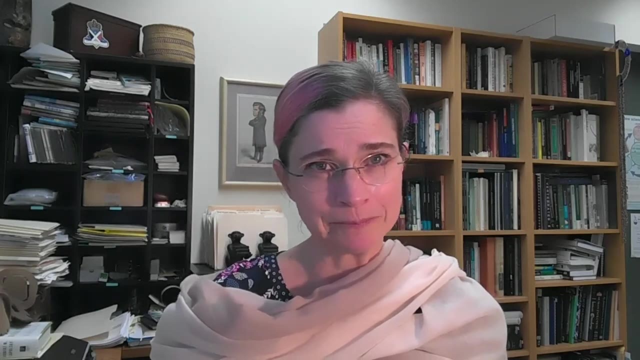 actually envisioned and created by scientists. about the science, This is a popular technology one. Now then you know the NASDAQ, for the best proof, tym Kneiger, and this is why I'm going to give you the porque. I think these videos are an excellent way to get introduced to some of the topics that we cover in this class. so 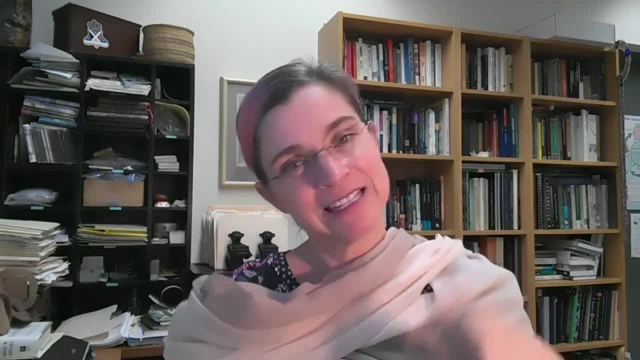 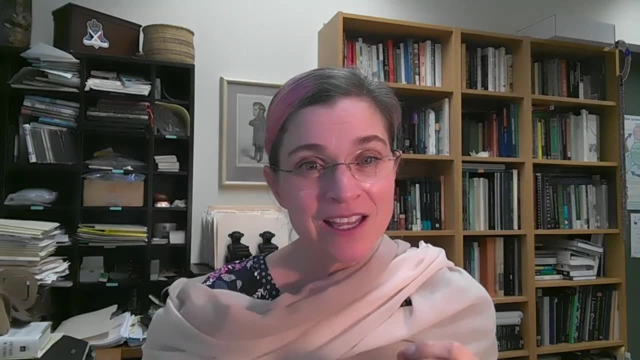 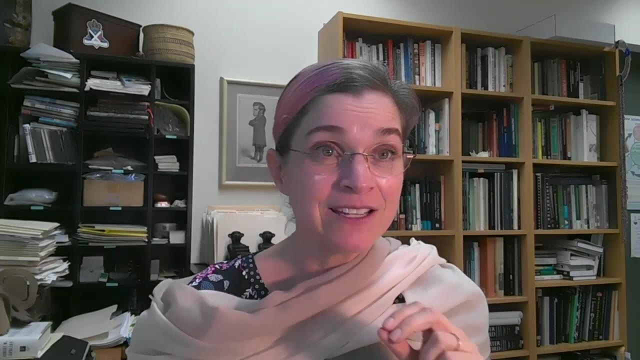 I'm going to have you watch a few of them over the course of this semester. Today I've set you up to watch one about human evolution. The glitch here is that this is my primary research area. strong opinions about how the science is presented, And however much I admire and 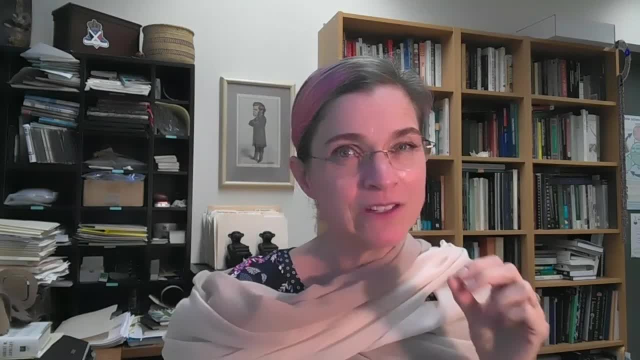 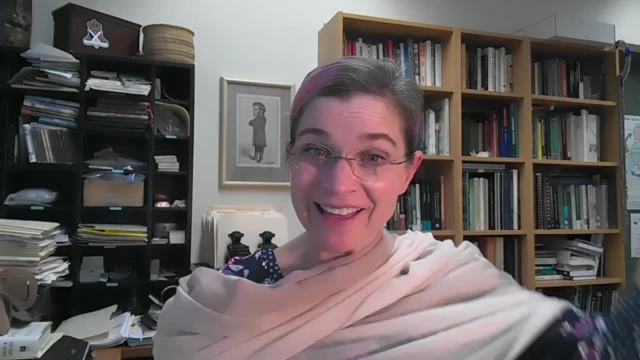 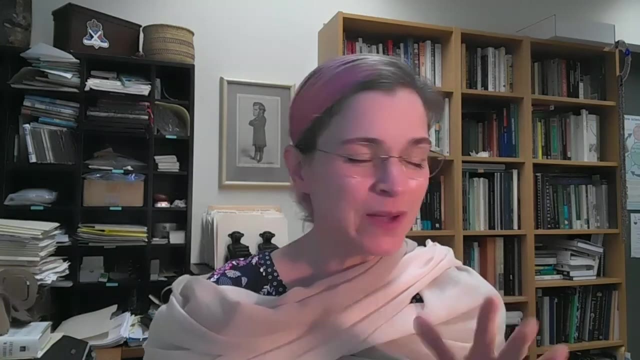 respect, Sean Carroll, if it had been me in charge, I'd have done this video a little bit differently, But thanks to Kaltura and Bcourses I can. So what we're gonna do is watch the beginning of the video and then, when it gets to where I think, 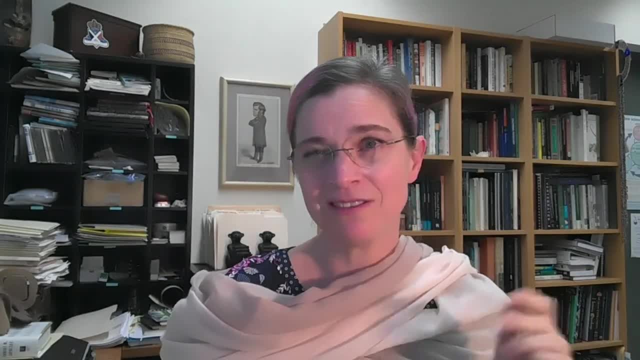 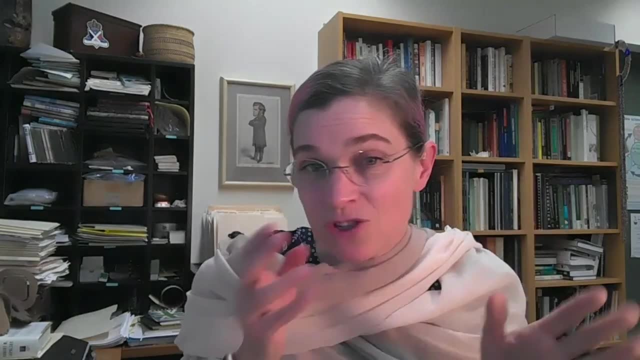 you'd be better off hearing some more recent research rather than the historical bits he focuses on. we're gonna cut away and I'll talk a little bit more and show you some photos, introduce you to some other researchers and then we'll go back and watch the rest of the HHMI video with Sean Carroll. 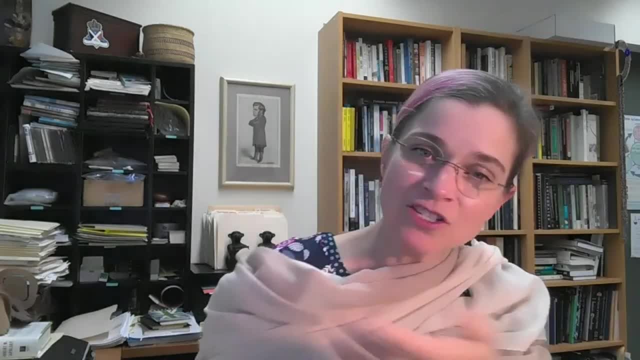 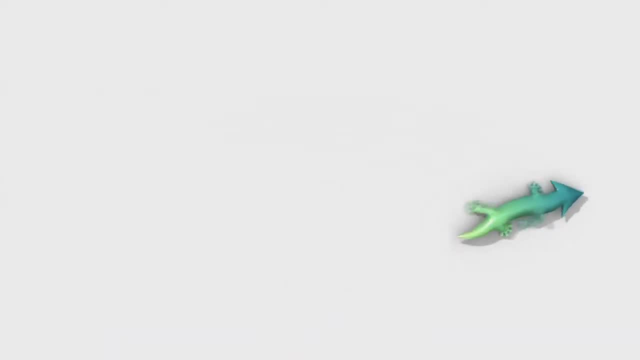 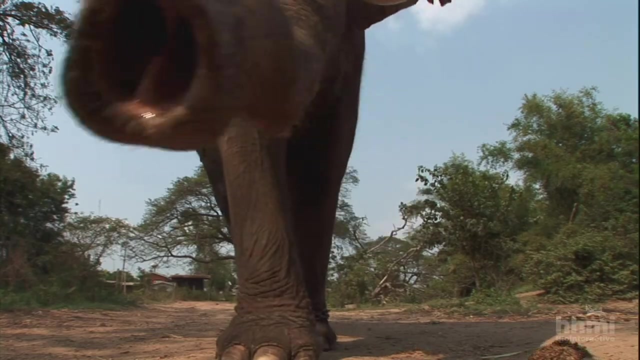 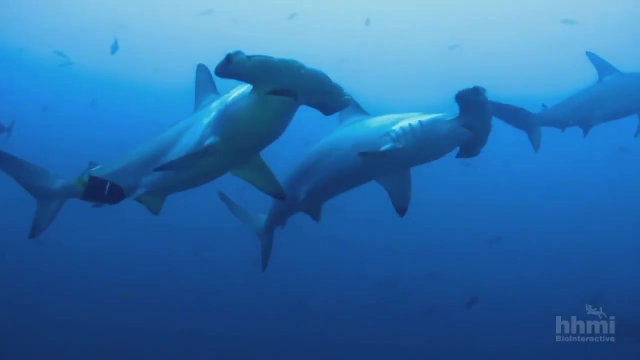 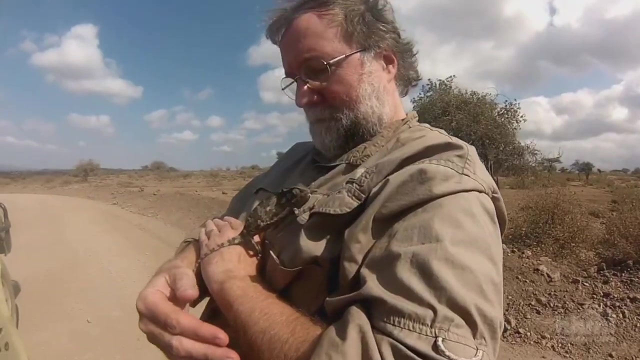 And so, with that, I pass you on to the HHMI video. See you in a few minutes. Explaining the origins of key traits that distinguish species has long been one of biology's fundamental quests. That's especially true for our own species, If 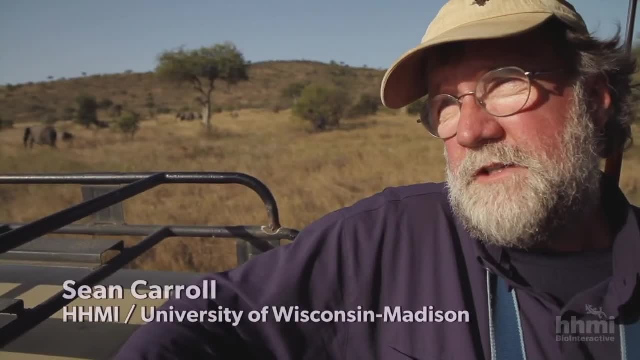 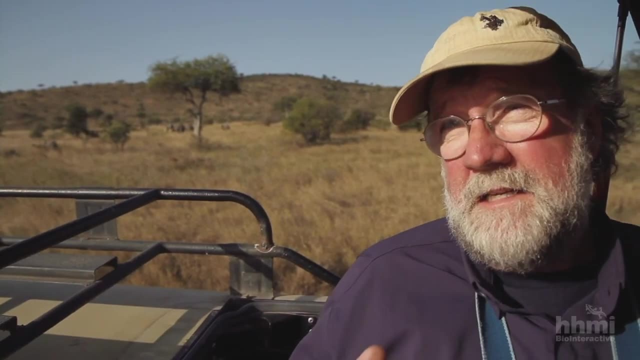 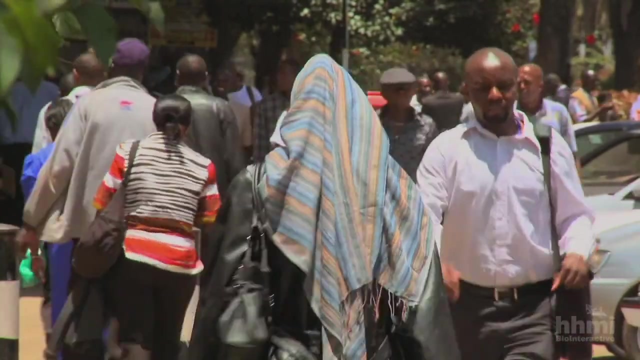 we look at humans as a biologist. with any animal, certain features stand out: Our big brains, The way we get around on two legs instead of four, and the way we use our free hands to make tools. Each of those three traits marks an enormous difference between us and our primate relatives. 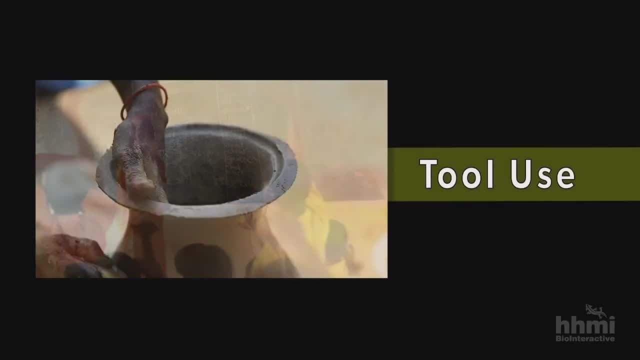 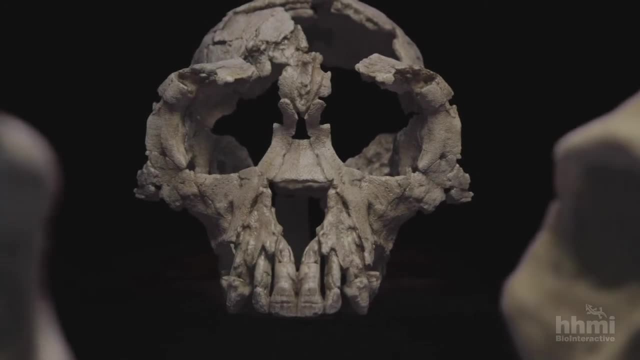 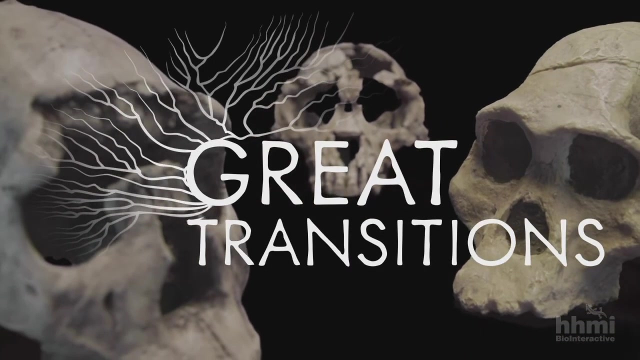 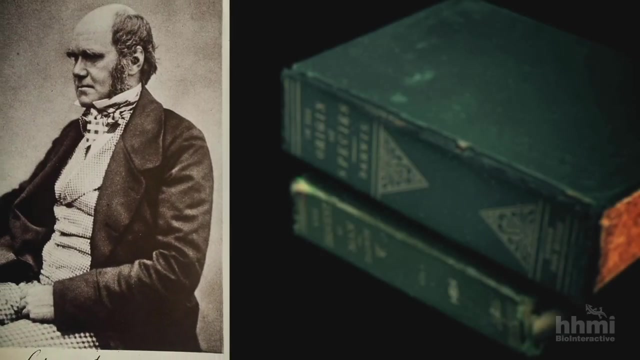 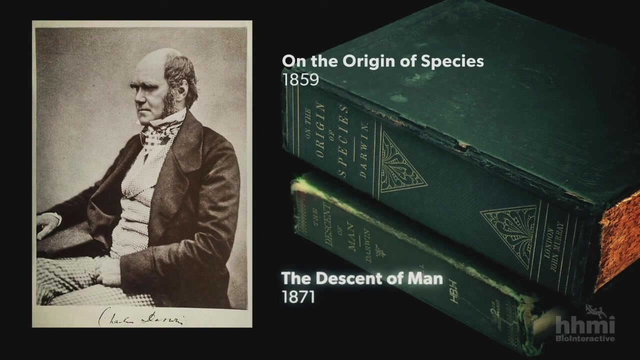 But when did they evolve, and in what order? The quest to understand our past has revealed much about the evolution of these features, All of them milestones in the great transition from apes to humans. It was many years after Charles Darwin had published his theory of evolution that he finally addressed the question: What about us? 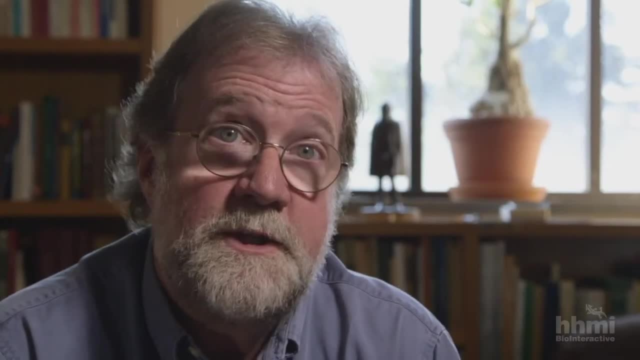 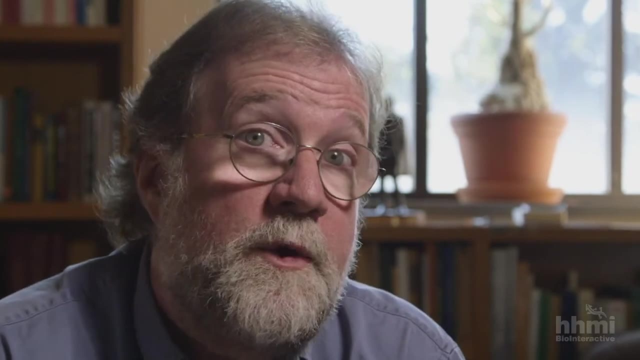 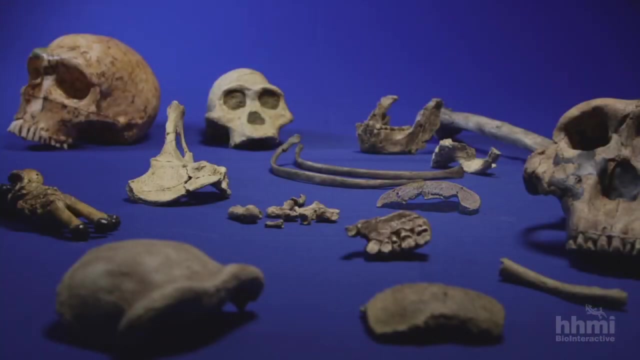 He speculated that we are descended from a common ancestor We share with African apes. the hope was that some geologists or paleontologists would one day Recover the fossils. that would settle the question. Fossils are essential evidence when putting together an evolutionary history, But in Darwin's day and for many decades after, few early human fossils had been found anywhere. 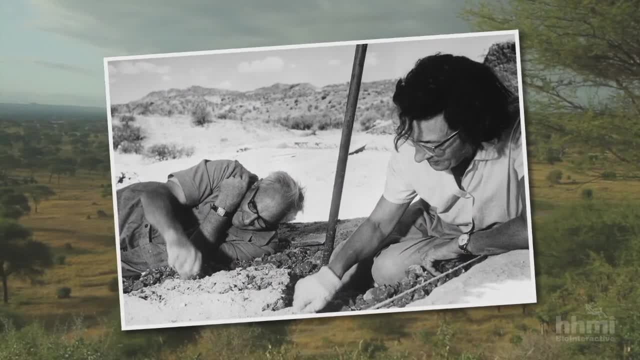 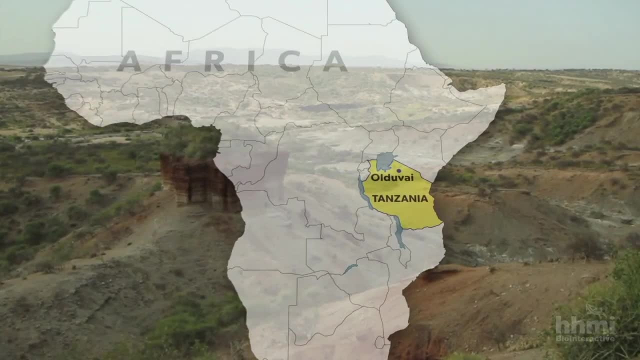 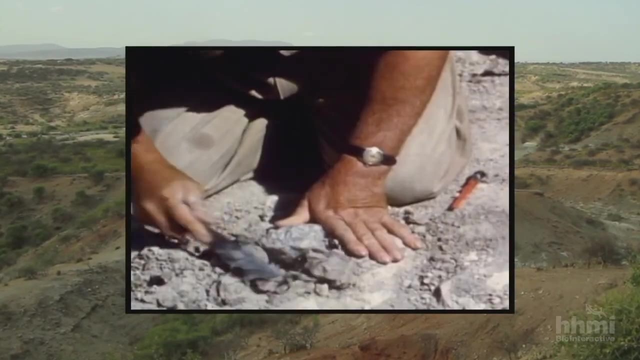 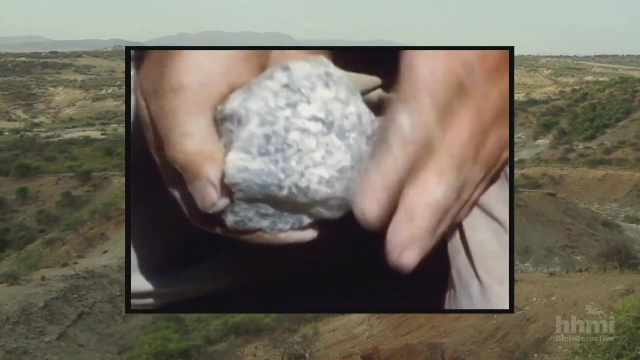 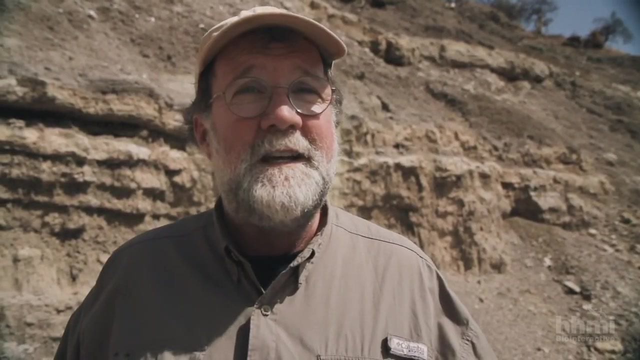 Anthropologist Lewis and Mary Leakey thought Darwin was right about Africa, So they searched for early human fossils in places like Tanzania's Olduvai Gorge and the Southern Mediterranean. Here they found abundant stone tools, But for the longest time the bones they sought eluded them. 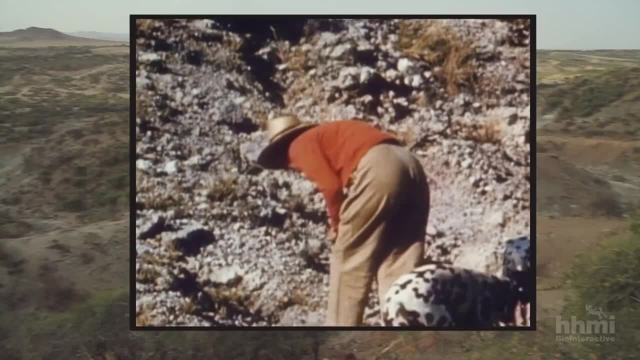 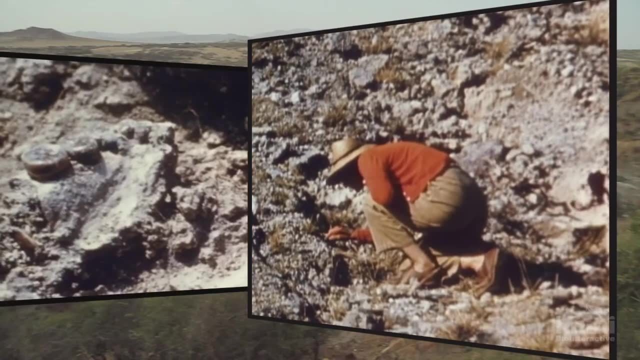 For almost three decades, all the leaky's found were tools, tools, tools everywhere, but not their makers. But all that finally changed. the morning of July 17, 1959, On a hill Mary had walked by countless times, something caught her eye. Poking through the eroding sediment was a huge upper jaw. 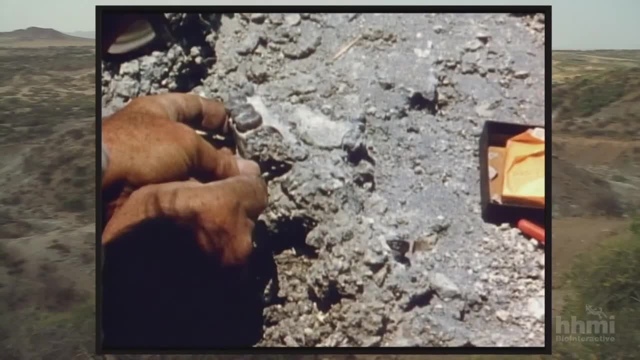 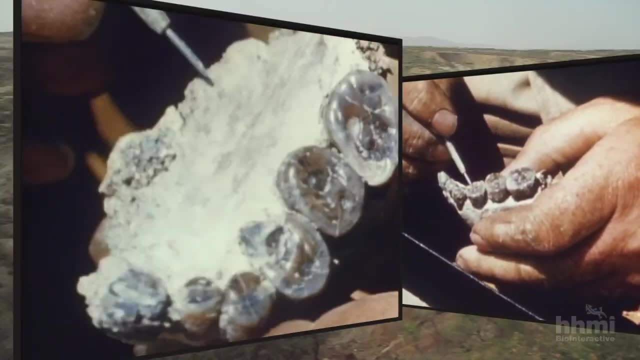 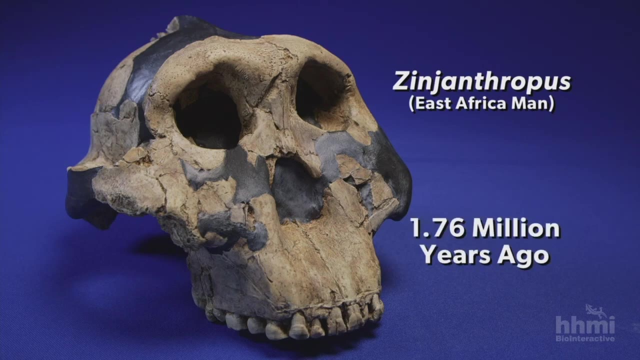 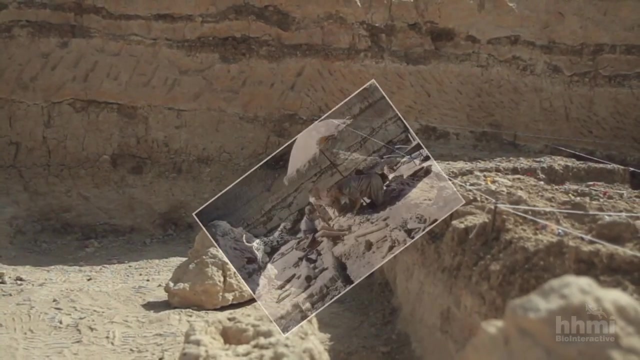 Together, she and Lewis carefully extracted bones from the skull of an early hominid. Geochemists analyzed the sediment layer it was buried in and determined this hominid had lived a stunning 1.76 million years ago. Remarkably, the very next year, the Leakeys 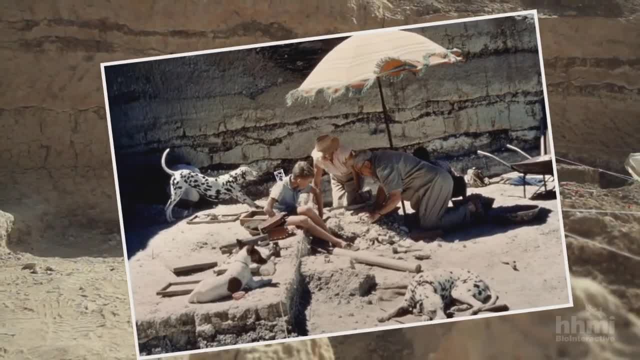 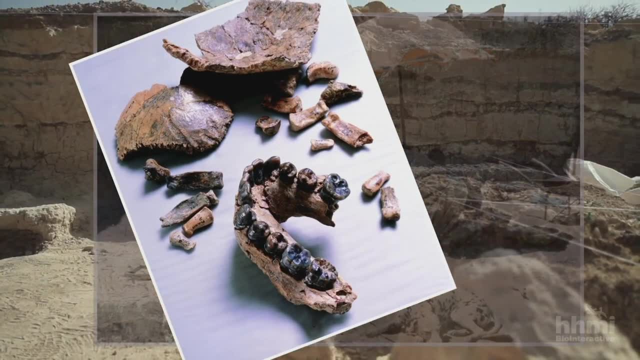 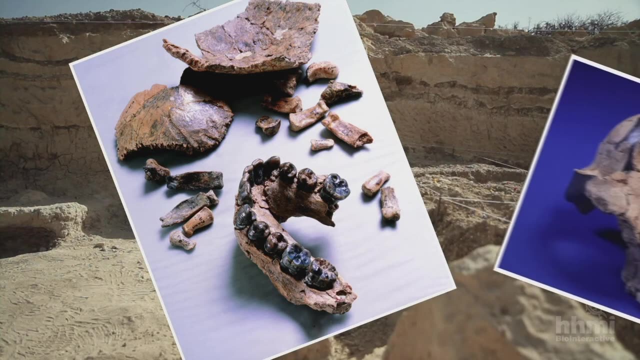 made another discovery. They designated it Olduvai, hominid number seven. It too was almost 1.8 million years old, But the recovered skull pieces and finger and wrist bones led them to conclude it was a separate species of early hominid. 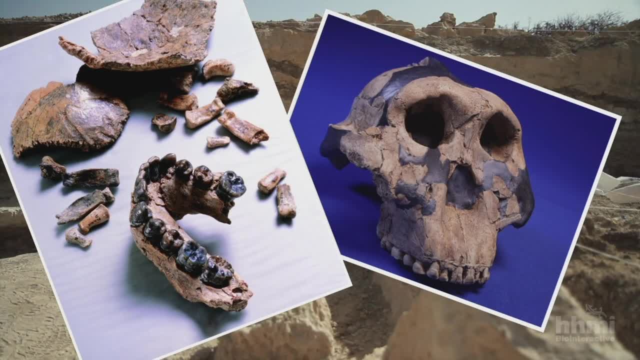 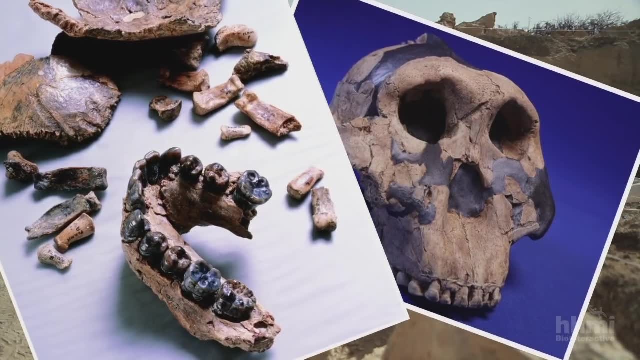 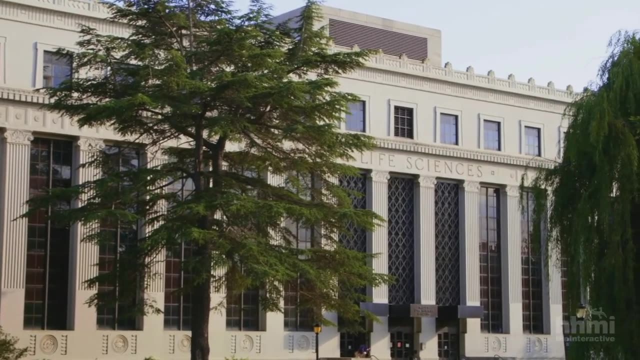 So there were at least two different evolving lineages of humans alive at this time. These discoveries helped swing the focus of human paleontology to Africa. Detailed casts of these and many other fossil finds are kept at the Human Evolution Research Center at the University of California at Berkeley. 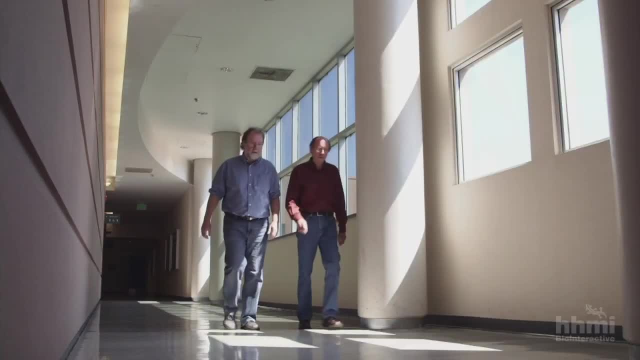 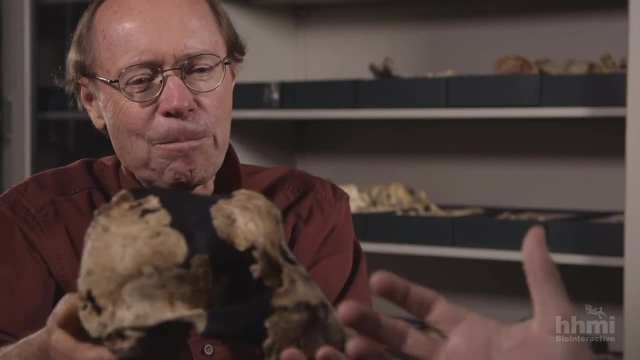 Dr Tim White, the center's director, has been involved with many of the important hominid discoveries of the past four decades. Clearly it was a hominid. I asked him what the current view is of the Leakeys'. 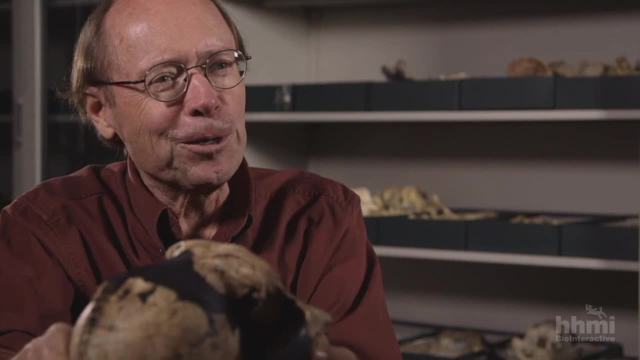 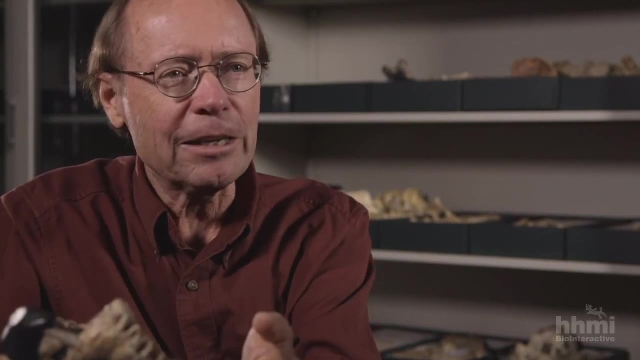 first discoveries. Well, I guess, after chasing the toolmaker for so many years, they initially thought, oh, we've found the toolmaker. But it turns out this large crest, the huge back teeth of this, show that it's on a side branch of human evolution. 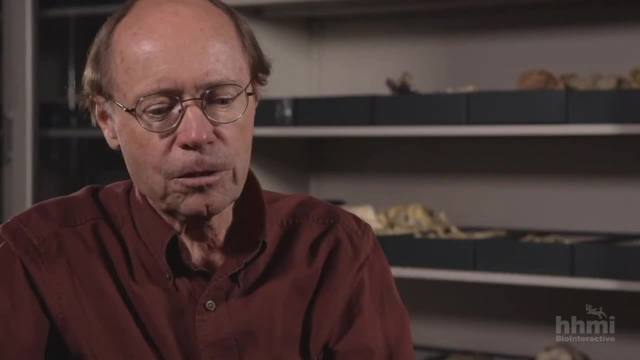 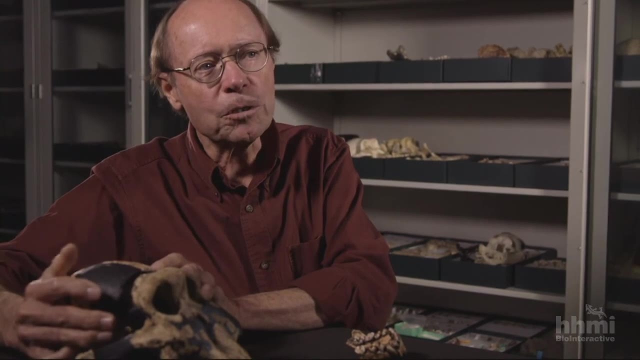 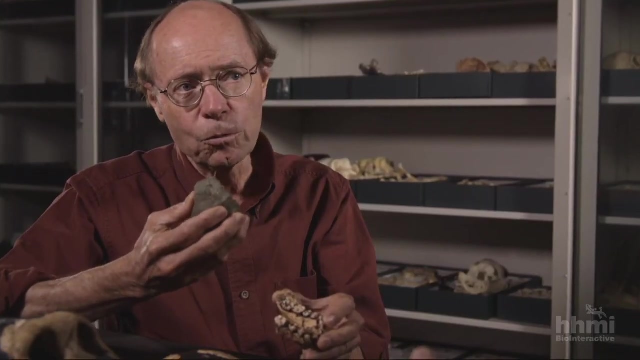 Probably not the toolmaker, But fortunately the next discovery was Olduvai hominid number seven, with a cranium much larger in size and a face much smaller in size, and probably the maker of these very primitive stone tools from the very bottom of Olduvai Gorge. 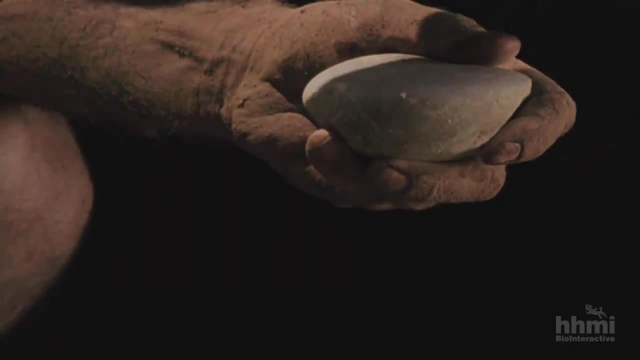 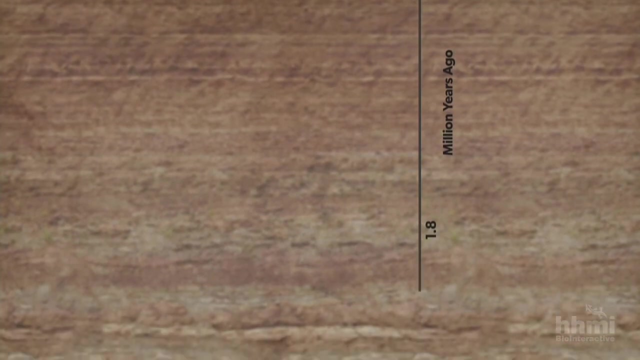 The early humans found at Olduvai were bipedal toolmakers with brains not as big as ours but larger than those of modern chimps, our closest primate relatives. So all of these traits must have evolved between 1.8 million. 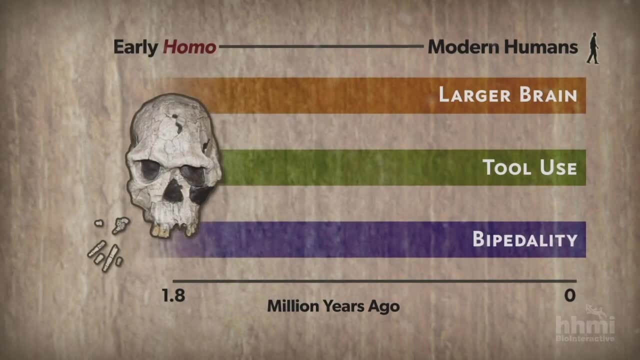 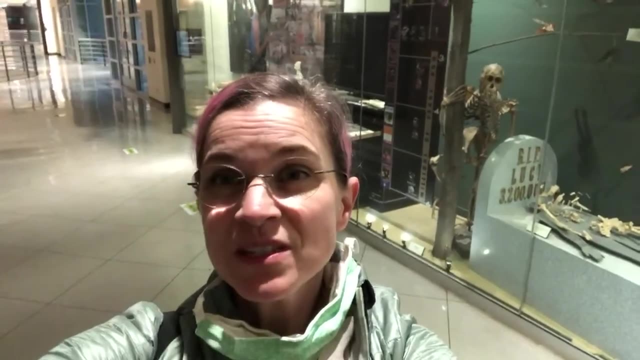 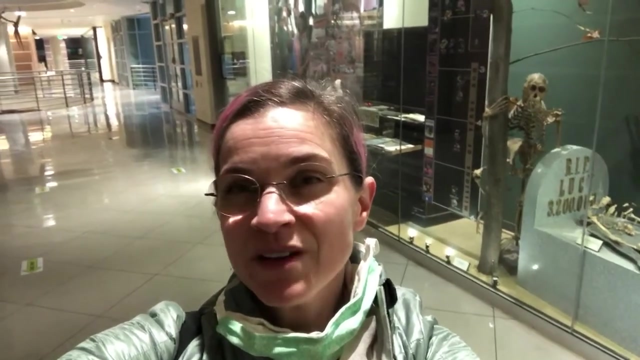 years ago and whenever the human and chimp line separated. You've just been introduced to Lewis and Mary Leakey and also Tim White. Now Professor White is a professor here at Berkeley. He's the current director of the Human Evolution Research Center. 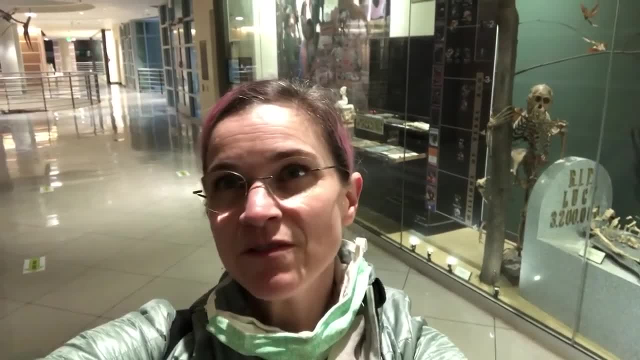 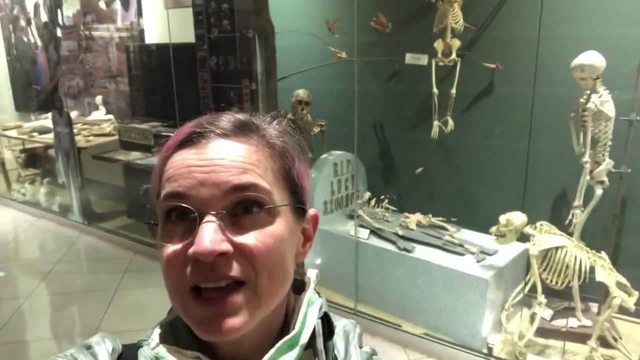 And he carries the torch of almost a century of human evolution research here at Berkeley. Now I'm standing in front of an exhibit here on campus, on the main floor of the Valley Life Sciences building. Now, when you are on campus, come check it out sometime. 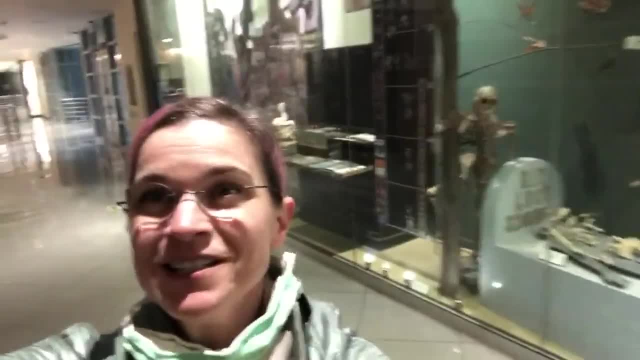 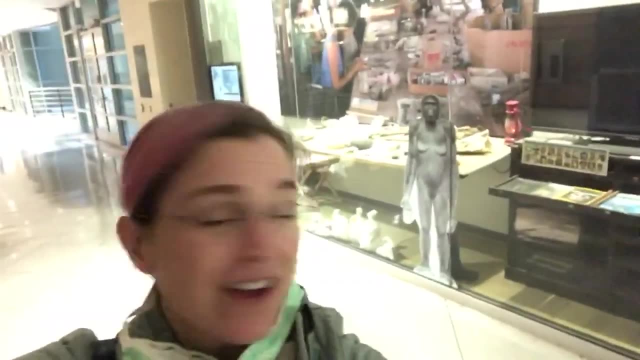 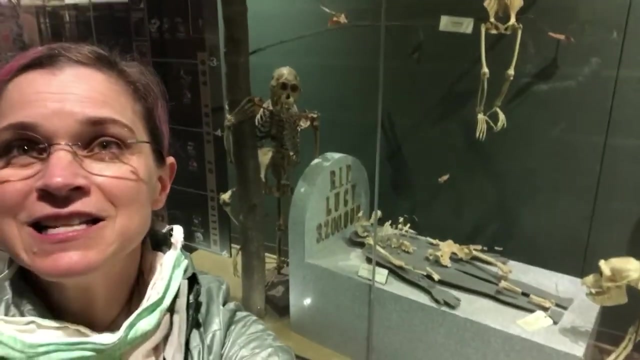 Now you'll get to see a reconstruction of a field. you get to see a reconstruction of a field camp and table. There is a cast of Ardi, of Australopithecus afarensis. This is Lucy, the skeleton there. 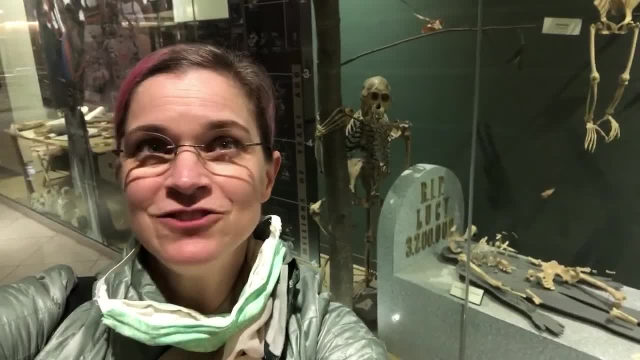 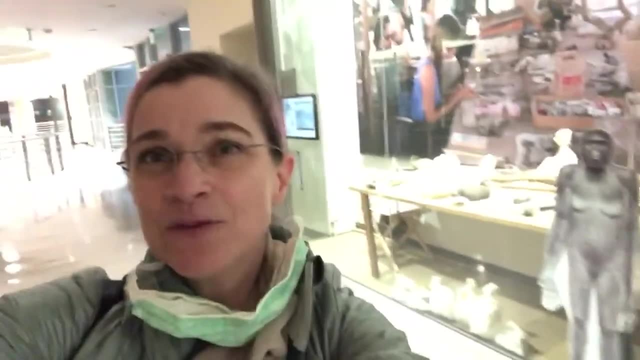 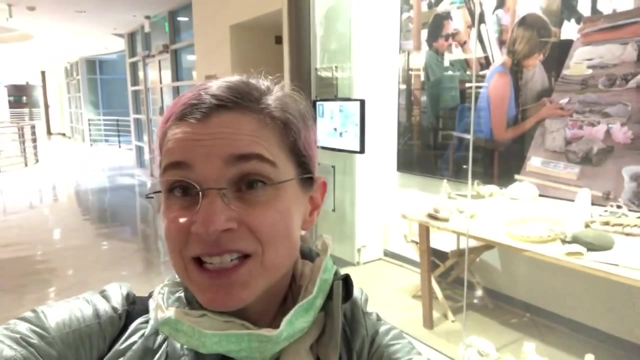 And you'll see her in the HHMI video in just a few minutes. And then there is also a slideshow of the Berkeley scientists who studied human evolution and who have studied human evolution here Now. two of the people in that video are Jackson and Zhao, and well me. 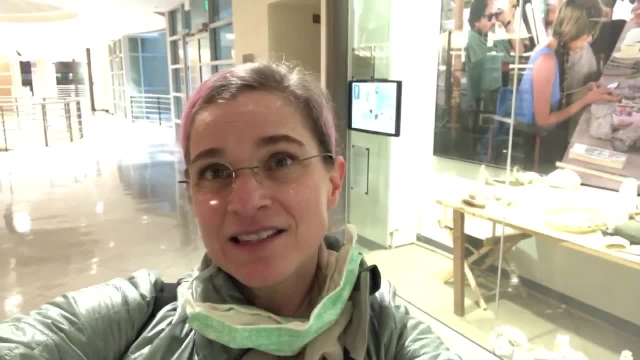 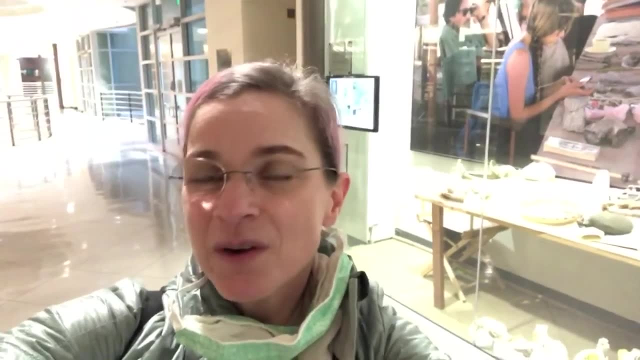 We've been working at Olduvai Gorge much more recently than the Leakeys, And since we are the Berkeley side of that story, I want to tell you a little bit about our work. And so now I'm going to switch over to PowerPoint for that one. 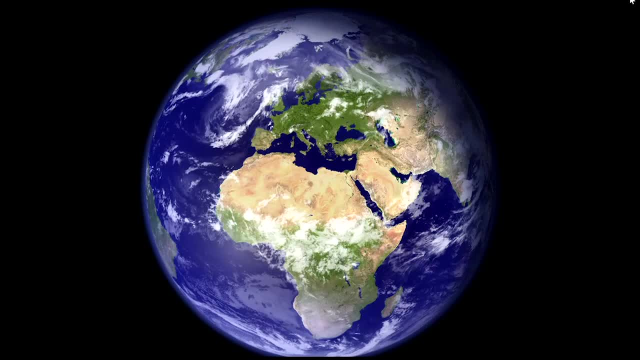 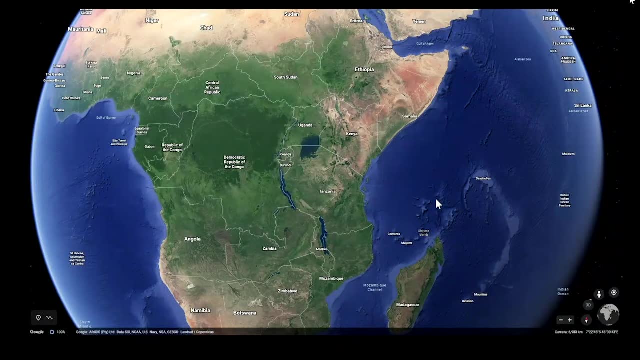 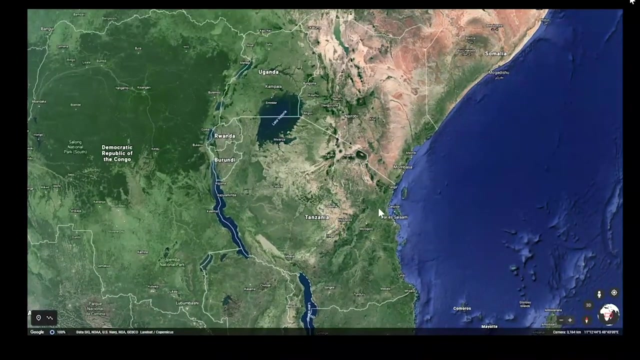 As you know from the HHMI video, Olduvai Gorge is in Tanzania, in Eastern Africa. Let's zoom in a little more. Let's zoom in a little more And then a lot more. The gorge is like a rip in the eastern edge of the Serengeti. 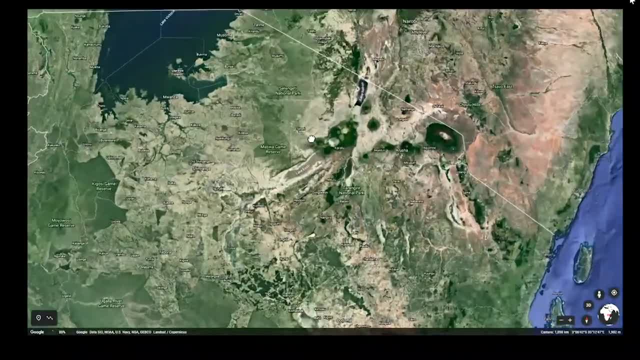 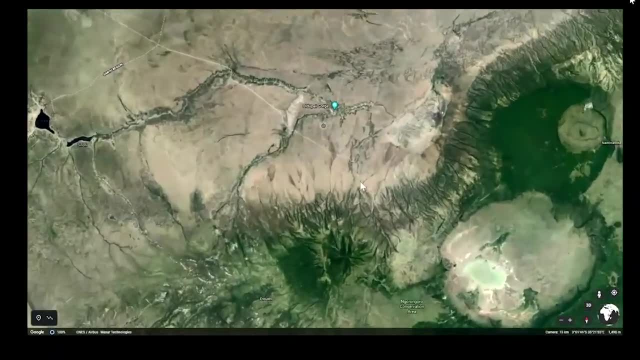 It exposes sediments that were deposited over the last two million years. So the Serengeti is to the west, which is left on your screen, And the Ngorongoro Crater is the giant green mass to the right. So we'll keep zooming in and spin around here a little bit. 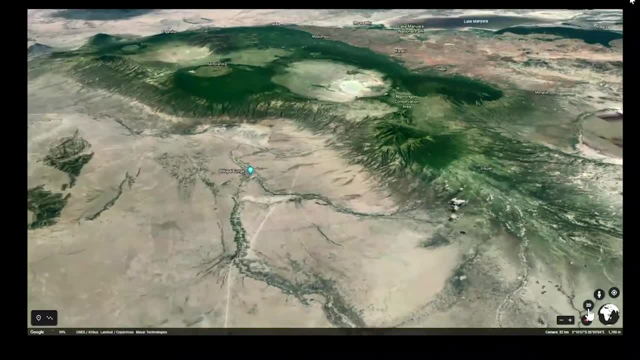 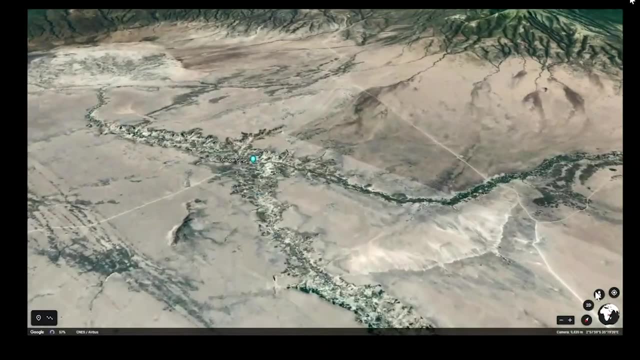 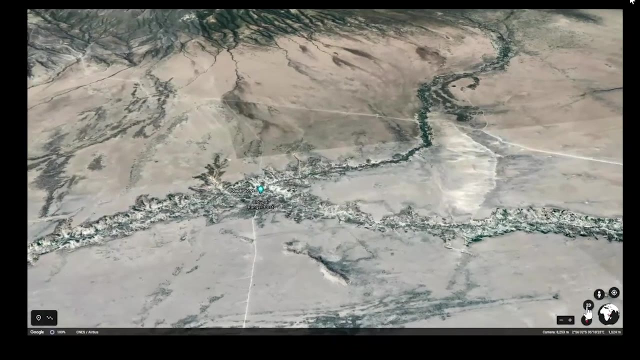 This is all done by hand. This is all done in Google Earth And I absolutely love Google Earth. I use it a lot in my field research, And now I'm going to draw you into this one area here, So you can see moving into 3D from 2D. 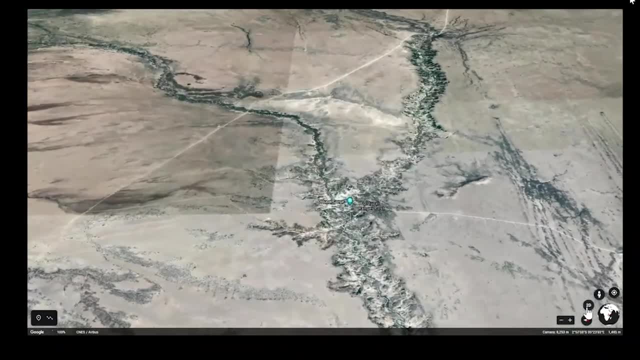 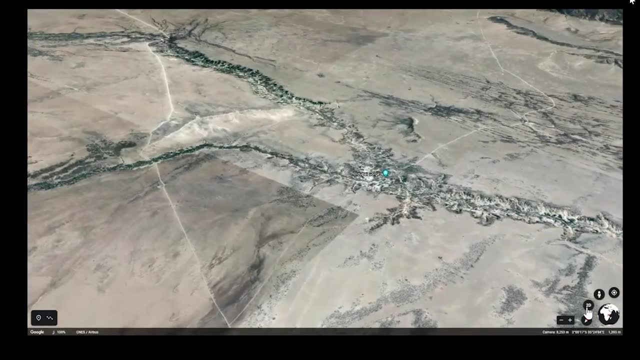 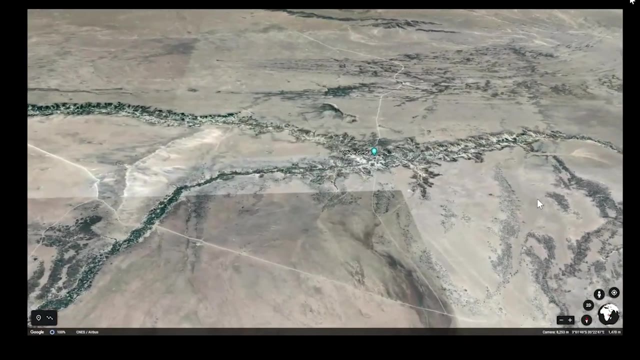 you can really get a sense of how it is: this erosional gully in a very, very flat area, the Serengeti Plain, So over on the right of your screen. there are these faults, And I want to draw you into one of them in particular. 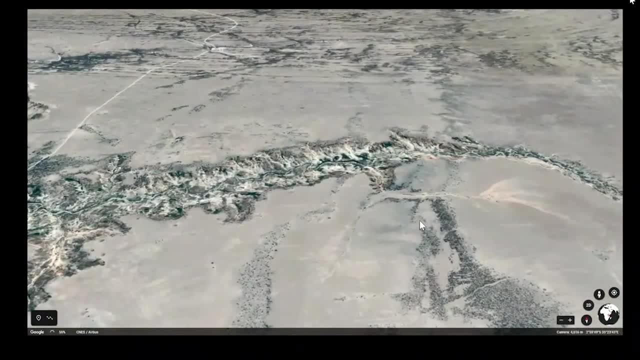 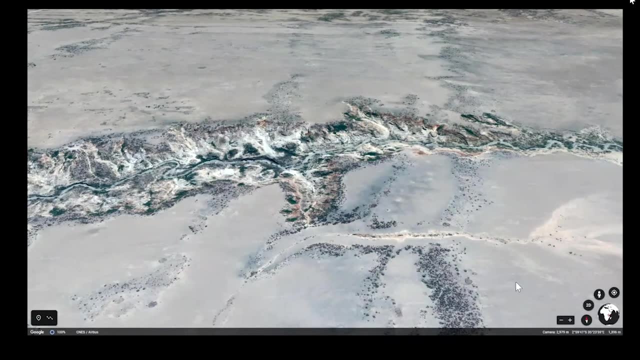 and kind of draw your attention to these orangish-reddish colors in the sediment. I'm going to pick this story up in a few minutes- right back on those red sediments. So draw your attention to that And then let's move on. 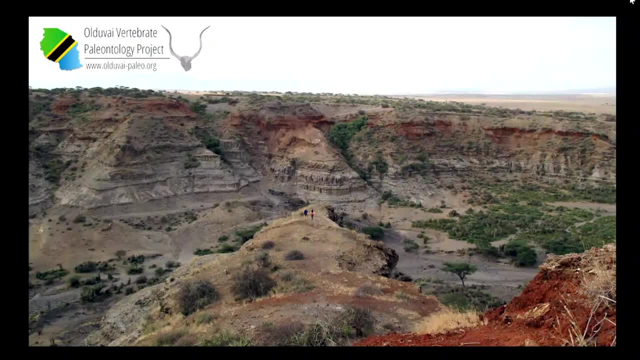 Jackson and Zhao and I co-direct a paleontological survey of the gorge. It's called the Olduvai Vertebrate Paleontology Project. We take our team out to survey for newly eroded fossils coming out from the sediments. Do you remember I pointed out those red sediments? 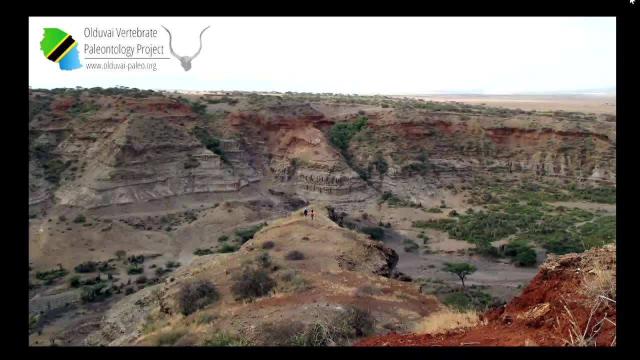 Well, here they are. from the ground perspective, And right in the middle of the screen, you'll see me standing there in my bright orange vest with another colleague on the project. It gives you a sense of scale. So here's Dr and Zhao. 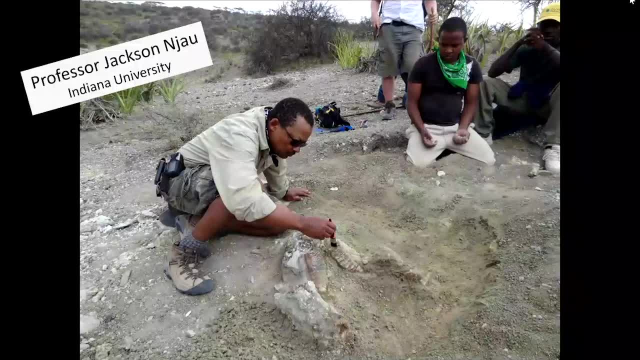 Professor Jackson and Zhao. he's at Indiana University excavating an elephant. the mandible of an elephant- Those are teeth, things that look like loaves of bread. That elephant was deposited in those sediments about 1.8 million years ago. 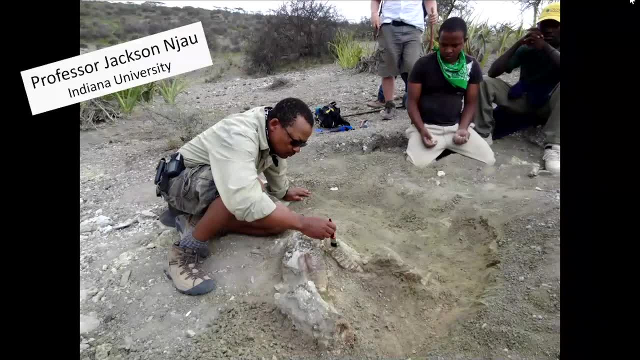 Those green tufts of plants. you can see them just between Jackson and the other people in the picture. those green plants are called olduvai bushes and they can get to be really big. In fact, olduvai the name, olduvai gorge. 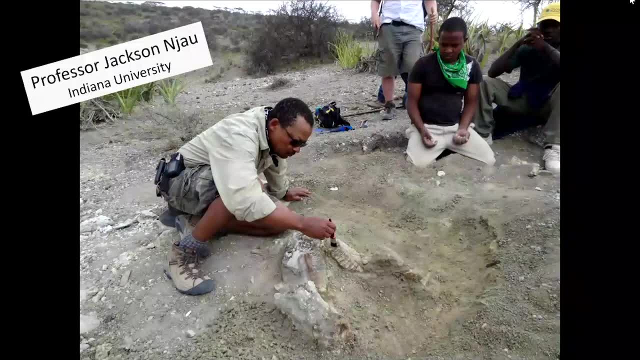 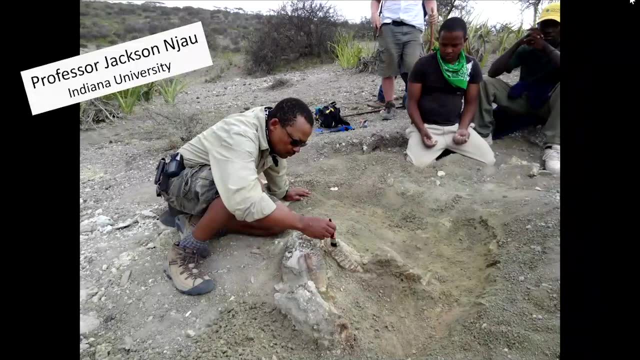 is supposed to actually be after the oldupai bushes, but it was mispronounced by the colonialists when they first started working there. So really, olduvai gorge should be called oldupai gorge with a P. We record very precisely using GPS. 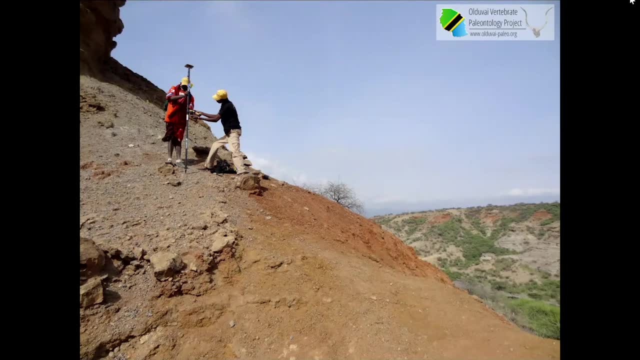 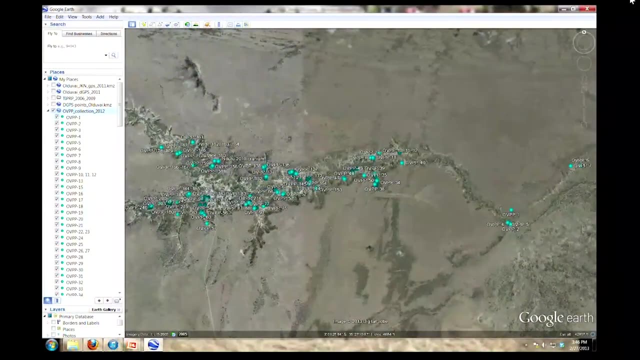 where each fossil is found. This enables us to keep very meticulous records of the dozens of fossils that we find each day in the field. Those GPS coordinates enable us to plot within centimeters exactly where fossils were found. Databases and imagery like this 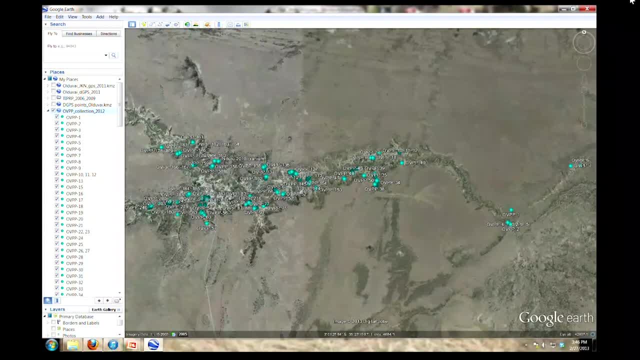 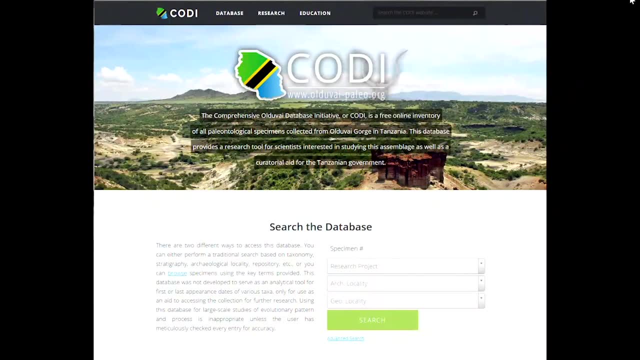 pretty standard practice in paleontology today. So each of those dots represents a plot of a fossil that we collected. We have all of the fossils inventoried into an online open access database that you are more than welcome to go check out. The URL is olduvai-paleoorg. 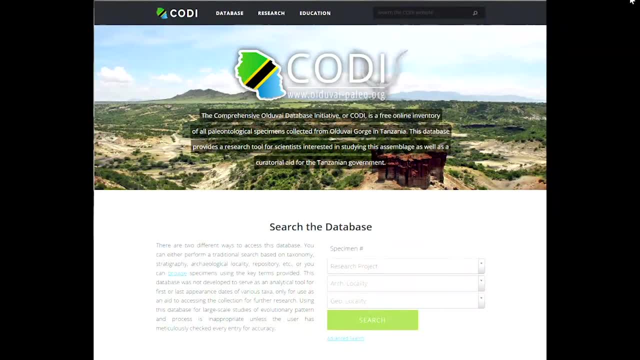 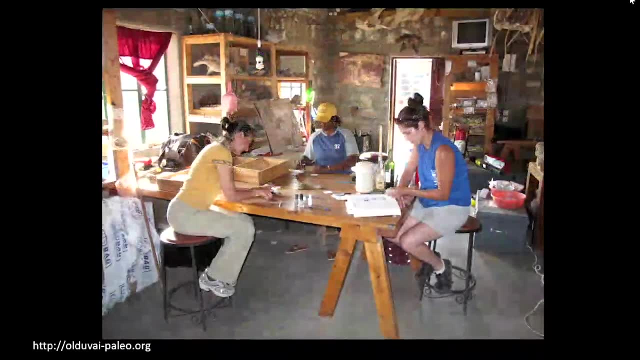 So all of the fossils that our project recovered are in this database, as well as all of the fossils that were collected by Lewis and Mary Leakey. This work takes a team and a few Berkeley students have had the opportunity to learn from the professionals in Tanzania. 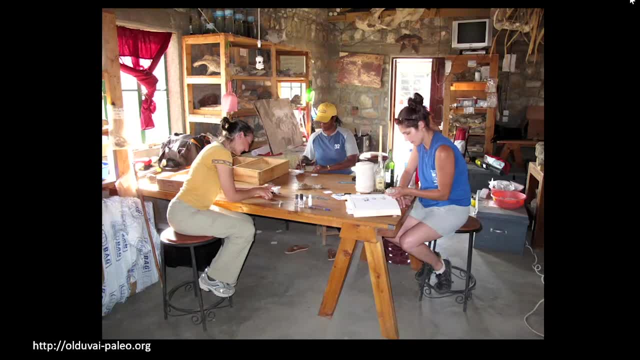 about fossil preparation and curation. On the right, you see a past PhD student in my lab. Her name's Whitney. She's now a data scientist, but during her grad school days she went with Jackson and I to Olduvai. 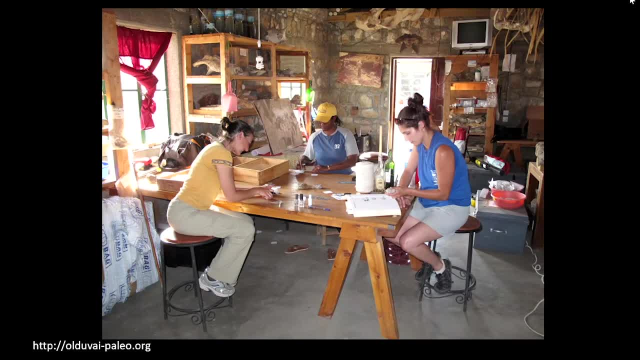 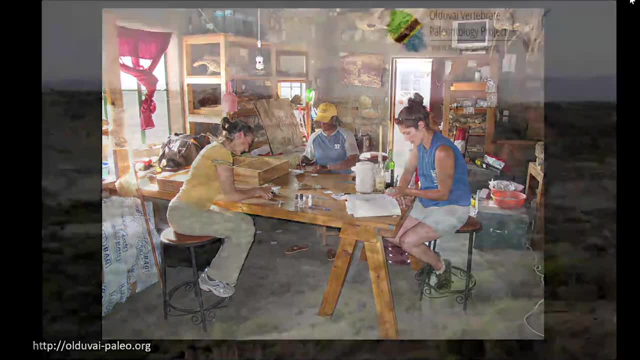 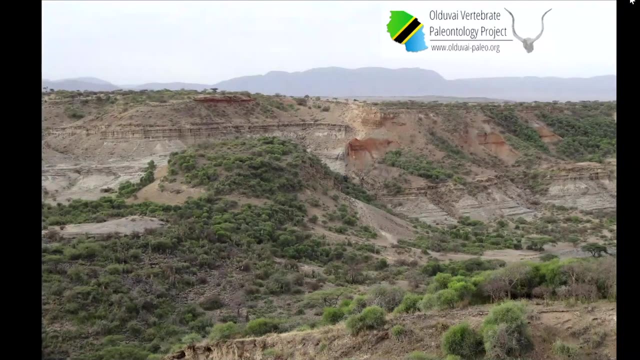 And here are people working in the lab out at Olduvai Gorge in one of the permanent buildings that are located at one of the base camps. On Whitney's second day at Olduvai, we decided to check out sediments exposed at this geological fault here. 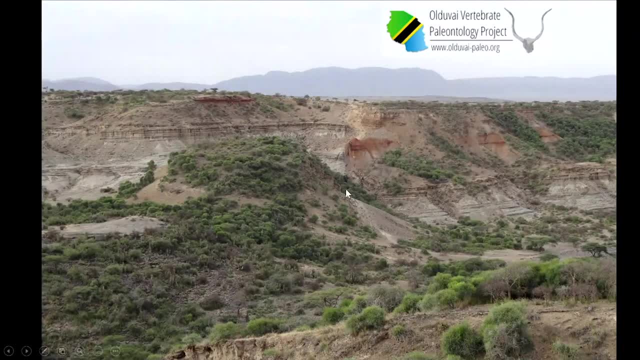 Let's see if I can show this here with my pointer. This is a fault right there, so the sediments go there and then they pick up over here. So you can see how there's an offset. So let me show you the car. 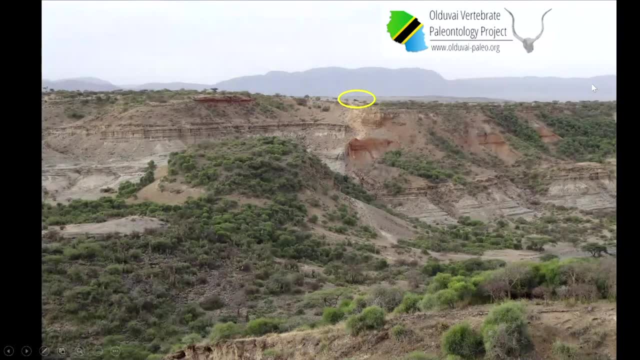 The yellow circle highlights our vehicle, to give you a sense of scale. So we hopped out of the car and started down the hill and just as we got to that red hill, right here, Whitney stops and shouts out: Hey, This looks like the ulna of a hominid. 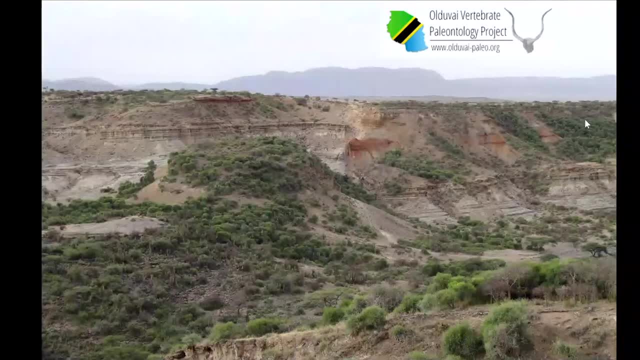 I walked over and all I could say was: Yep, sure does. The ulna is a bone in your forearm and the fragment that Whitney found is part of the wrist. Here's that fossil. It's the bone in the middle. 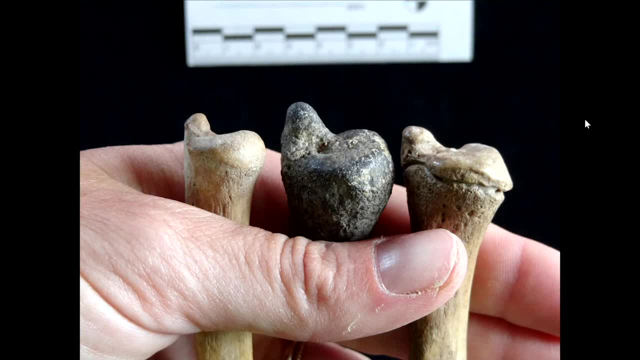 and it's darker because of the mineralization that happens during fossilization. Those are modern human bones on either side, Modern human ulnae. This bone is over one million years in age and yet it looks identical, essentially, to modern humans. 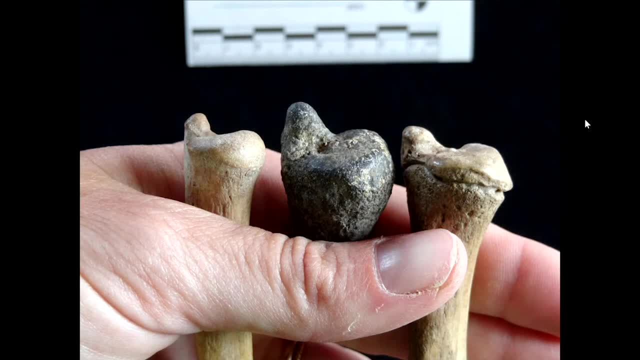 So one of the things out of this story is just to point out that field- paleontology- it's never that easy. Just that one time has it ever been that easy for someone to find such a rare fossil. But there you go. Okay, now let's get you back. 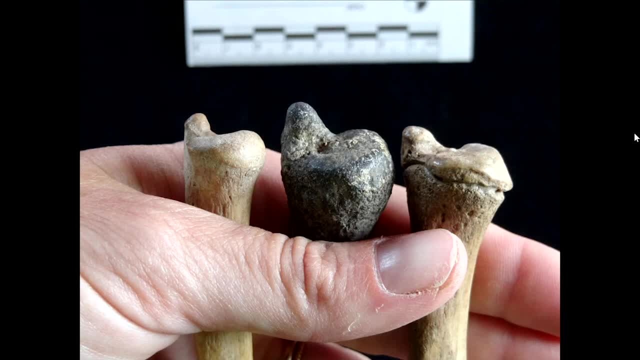 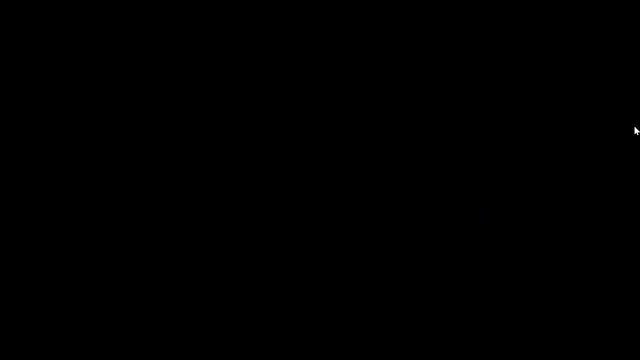 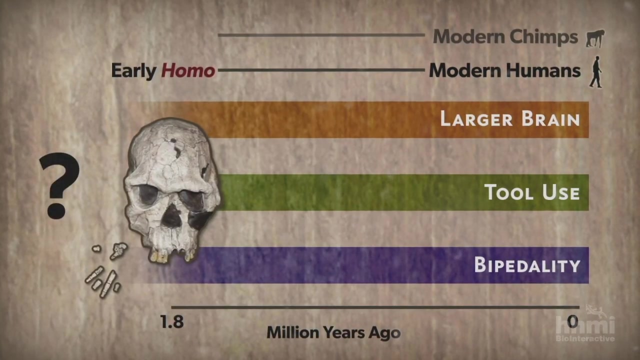 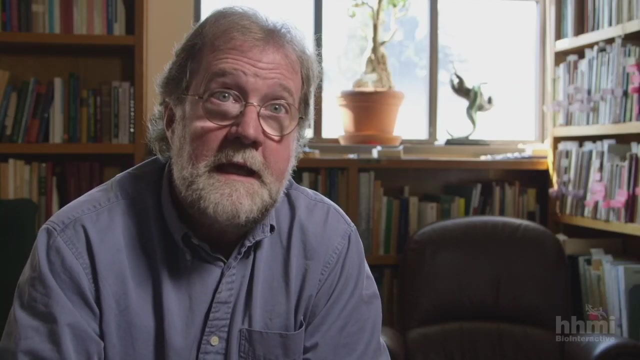 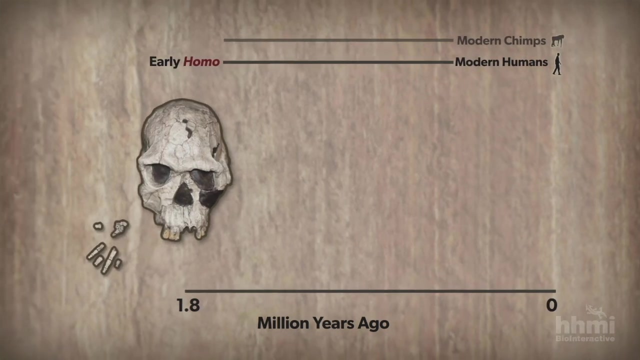 to the HHMI video. And when did that happen? At that point no one could say. But then Alan Wilson and colleagues here at Berkeley developed a revolutionary new way to use biomolecules, including DNA, to estimate the time of that split. 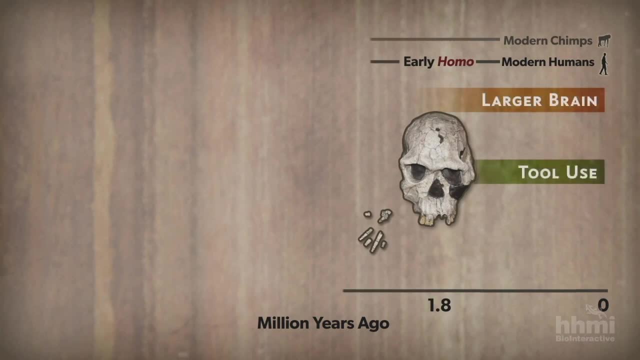 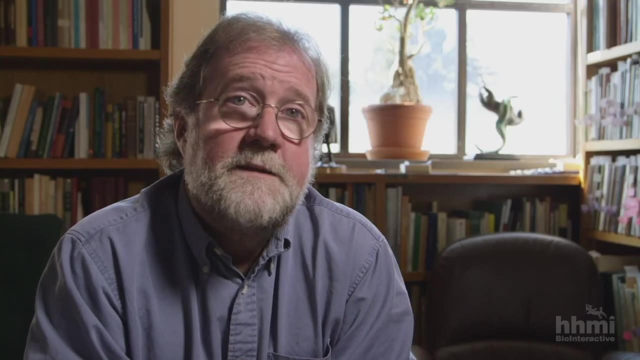 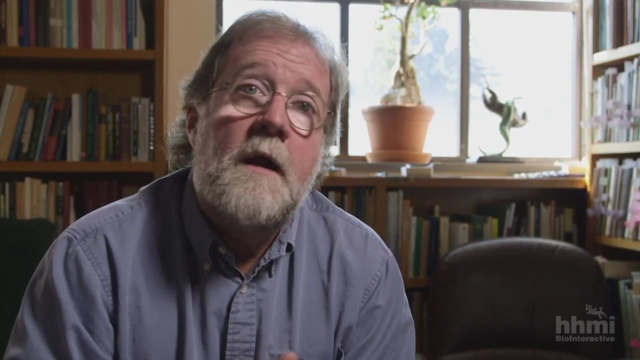 Using this approach, researchers have estimated that humans and chimps have been evolving independently for almost seven million years. DNA tells us that our lineage goes back several million years before the Olduvai fossils. What DNA can't tell us is where and when the traits that distinguish us. 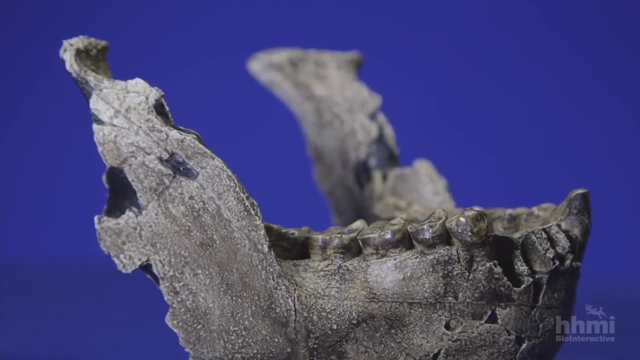 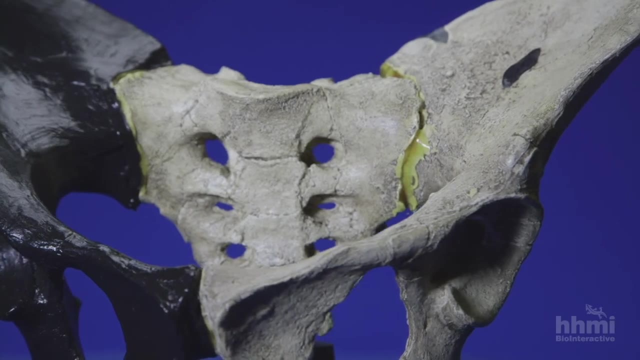 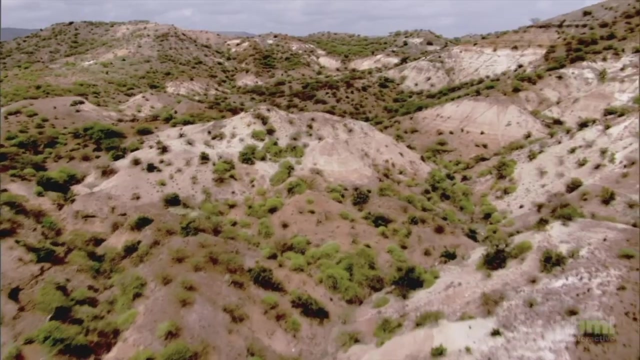 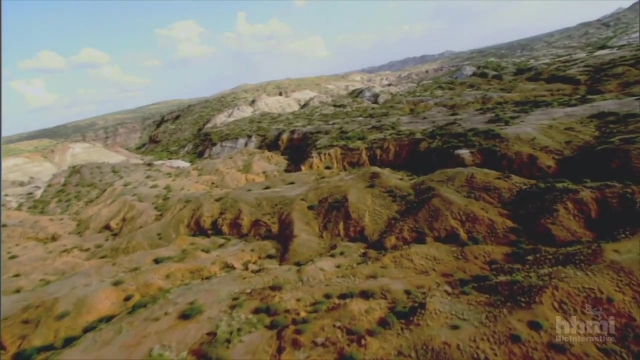 like bipedality first emerged? Only fossils and their ancient environments can address those questions. Eastern Africa is a fossil treasure trove because of the geological forces that have created the rift valleys that scar the region Over the eons- volcanoes associated with this rifting. 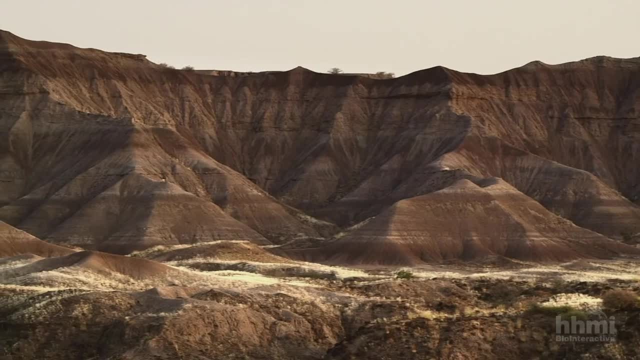 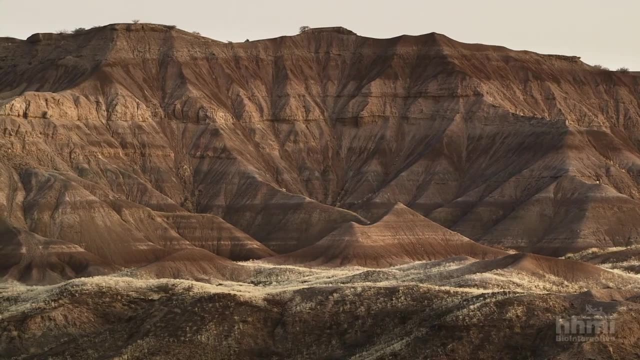 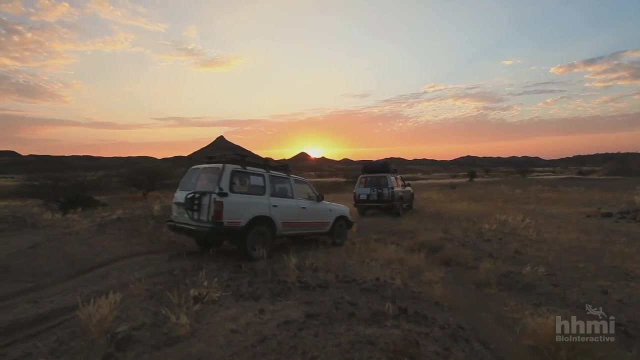 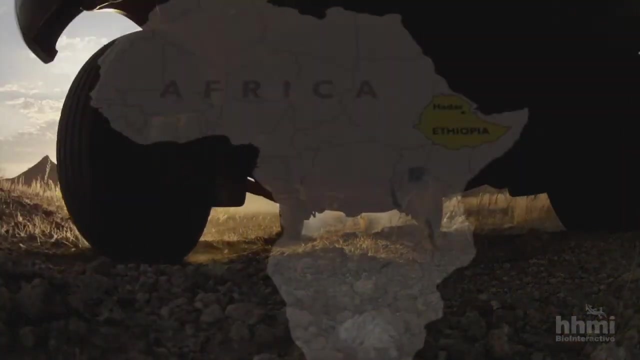 regularly blanketed the region with ash that included radioactive elements, the steady decay of which allows geologists to accurately date sediment layers and the fossils within them. Paleontologist Don Johanson remembers vividly the first time he visited the Hadar region of Ethiopia. 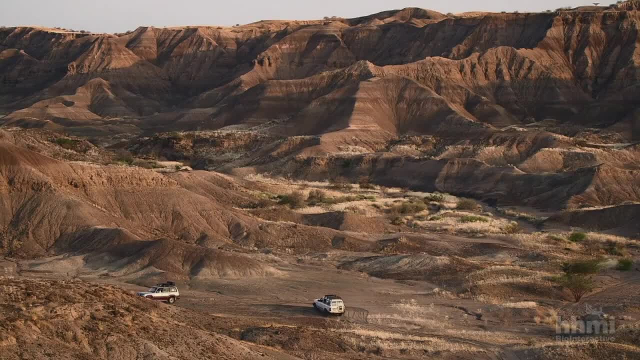 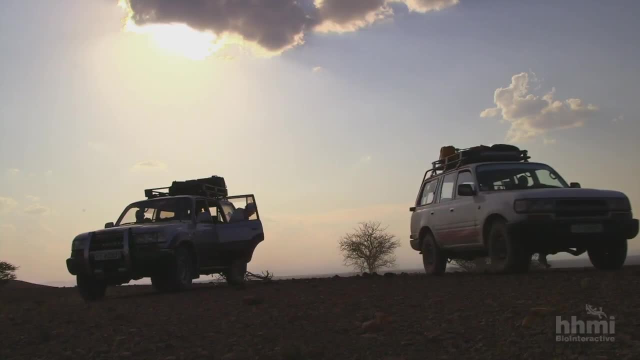 A thousand miles north of Olduvai, it has exposed sediments that are over a million years older. We drove up to the edge of this escarpment and it just unfolded, and there it was- All of the sediments getting deeper. 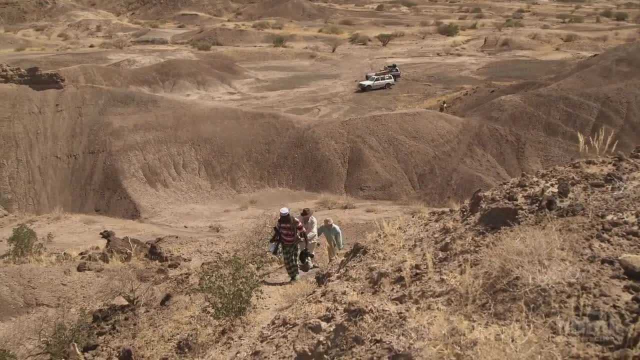 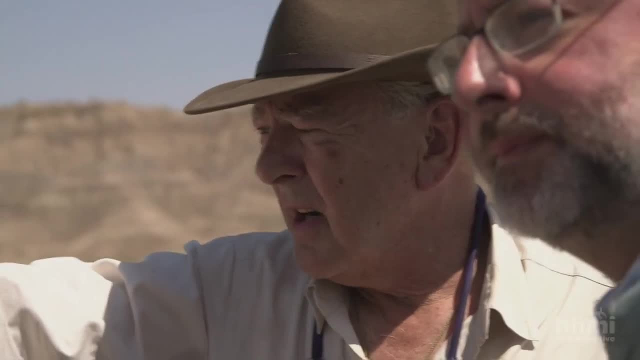 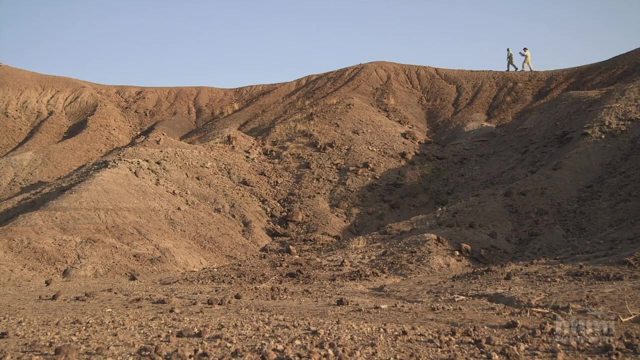 and deeper and deeper. I could not wait to get down there. The driving force was: find something, And then we walked out there. Johanson recently shared with fellow paleontologist Neil Shubin his memories of the day he discovered the first small bone fragment. 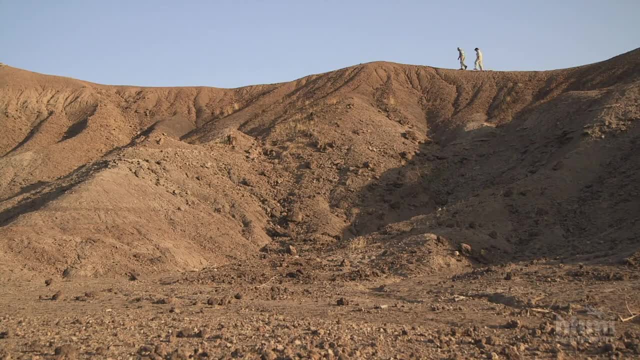 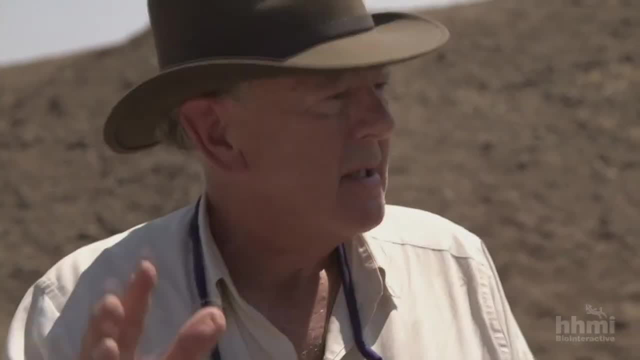 of one of the most famous fossil skeletons ever found. You know, my best recollection is that it was right in this area And I looked at it and almost instantaneously said that's a hominid. Just a fragment of elbow that led to the skeleton. 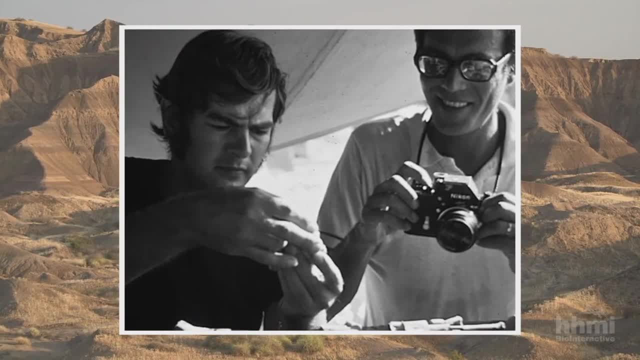 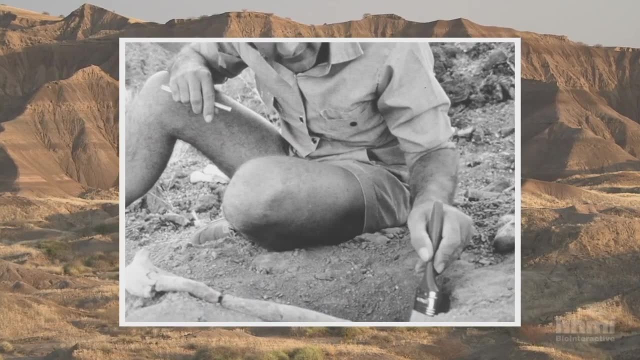 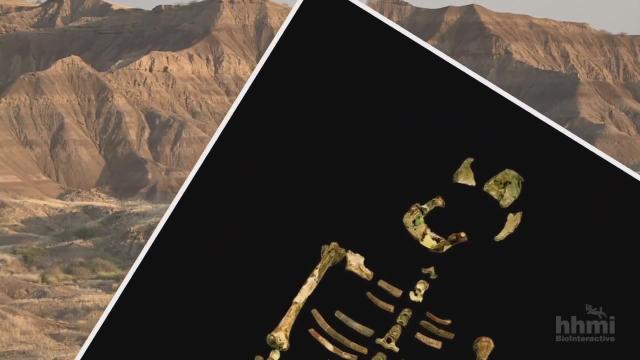 An international team of scientists helped Johanson recover almost half the bones of an individual who had lived 3.2 million years ago. They called her Lucy. Finding Lucy was really the first step in this very long process of description, investigation, evaluation. 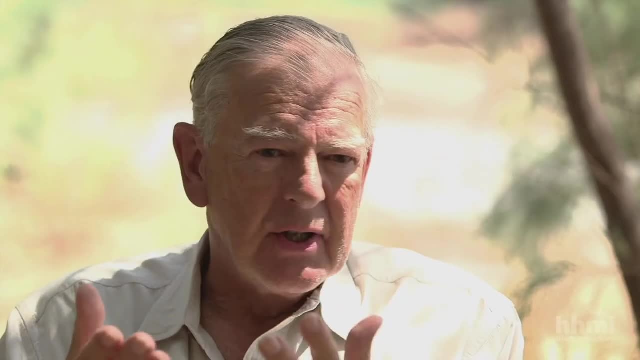 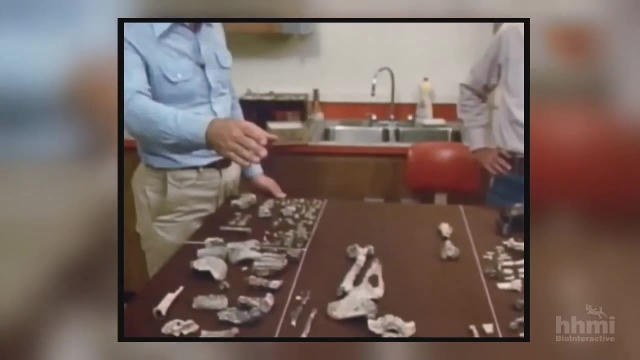 hypothesis testing, trying to figure out where in the world she sat. like we are on the tree, on the human family tree. Hey, sorry to interrupt again, but I just had to interject in this because I have a lot of questions that I want to ask you about. 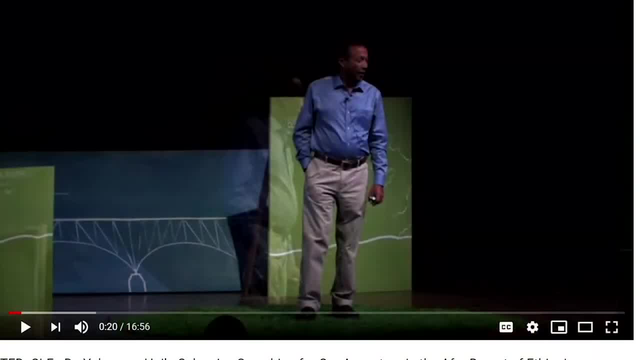 So I'm going to ask you a question about Lucy, But I just had to interject in this part Our knowledge of Australopithecus afarensis. it's increased so much since Lucy, And most of that's due to the spectacular research. 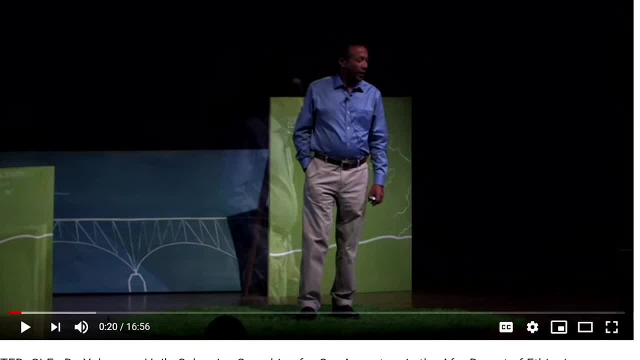 of two scientists leading research in the Afar these days, And both of them are Ethiopian paleontologists. So I want to introduce you to both of those just really quickly. The first one is Dr Johannes Haile Selassie, and he is a curator at the Cleveland. 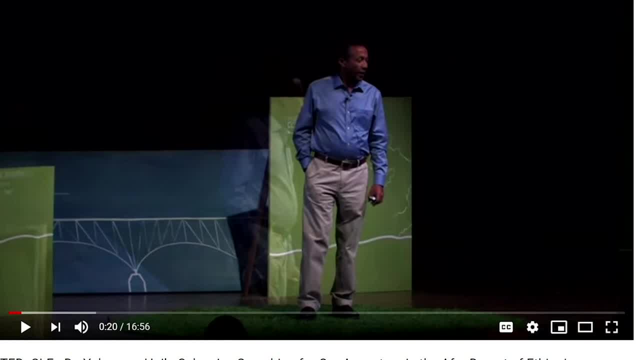 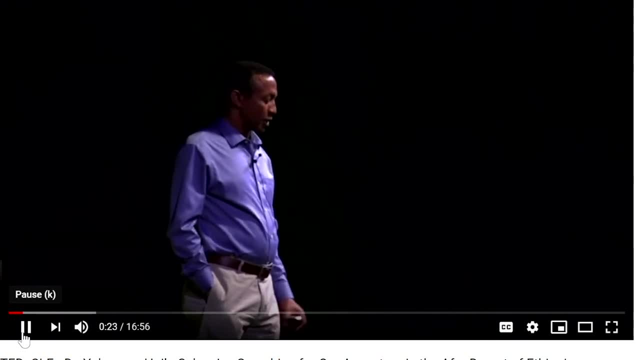 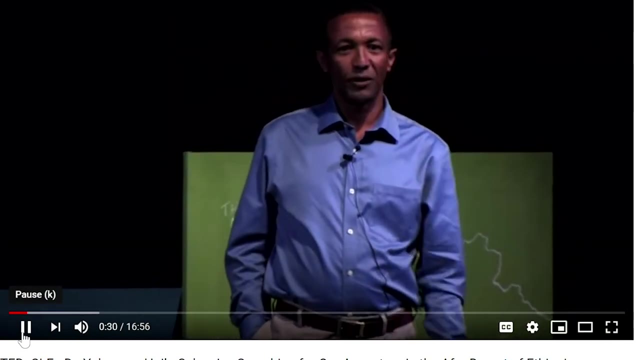 Museum of Natural History. So let me play a little bit for you of him talking about his own work. I'm a curator at the Cleveland Museum of Natural History next door, But most of what I do is paleontological field and laboratory research. 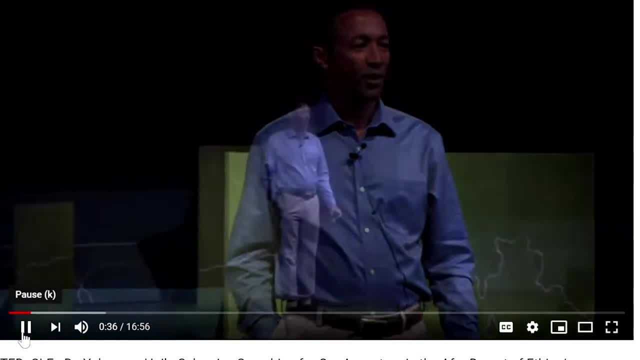 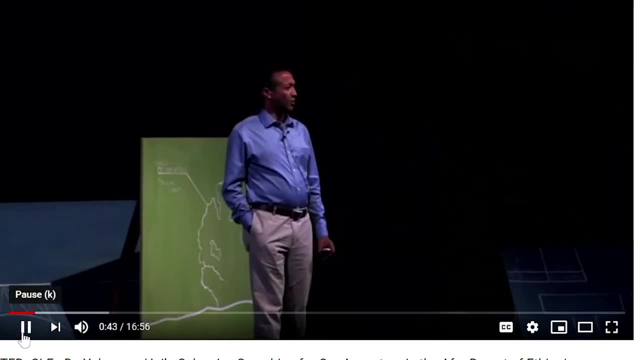 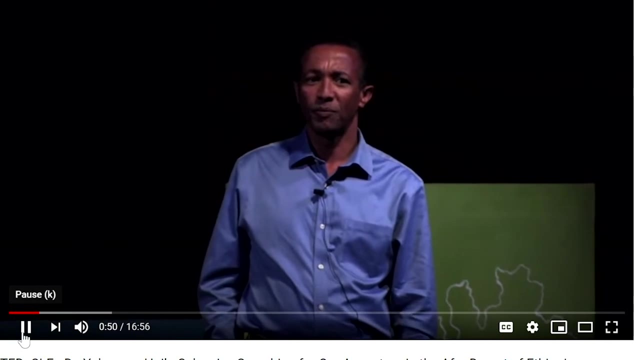 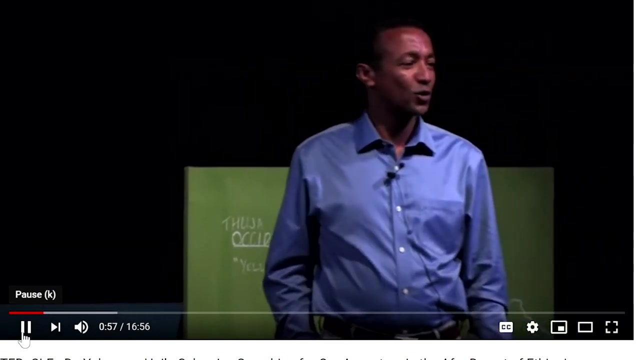 in an attempt to address one profound question, A question that each of you may have in mind, Very simple to spell out but extremely difficult to answer: Where did we come from? I've been trying to address this question for the last 20 years by going to very remote 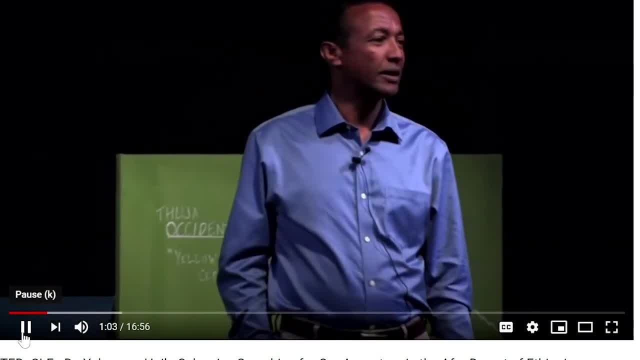 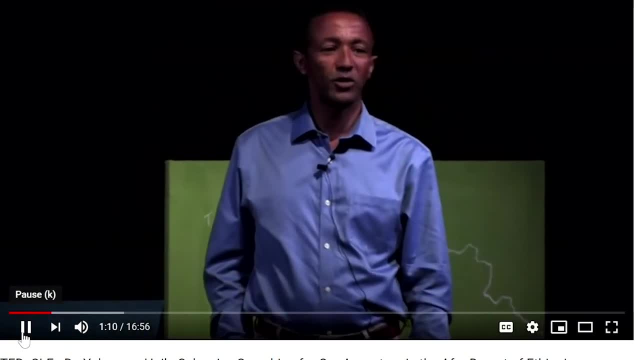 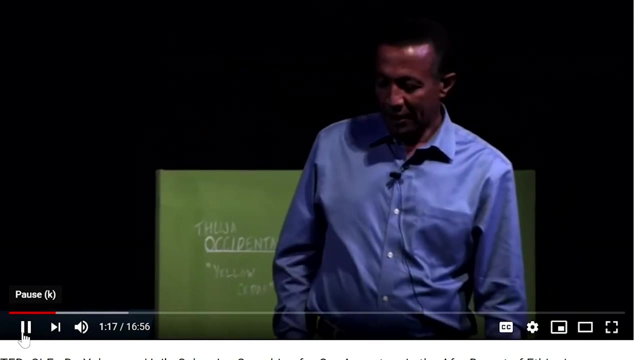 sometimes hostile area in Eastern Africa, in search of fossils that are, at least for us paleoanthropologists, our only clues to address the question of where we came from. Now, this area, this remote area that I'm talking about, is located in Ethiopia, which is right here, And the Afar Desert has been there for many, many years. It's a desert now, but millions of years ago this place was very lush, green, a lot of water and a lot of life. 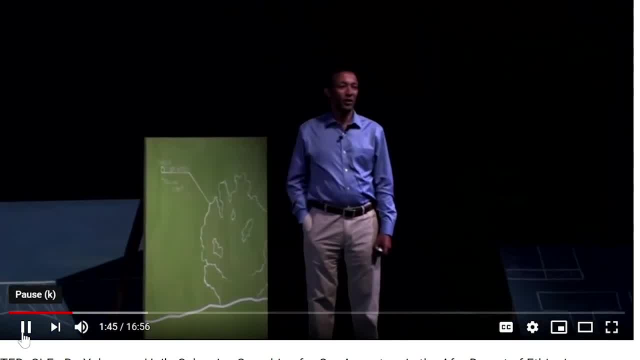 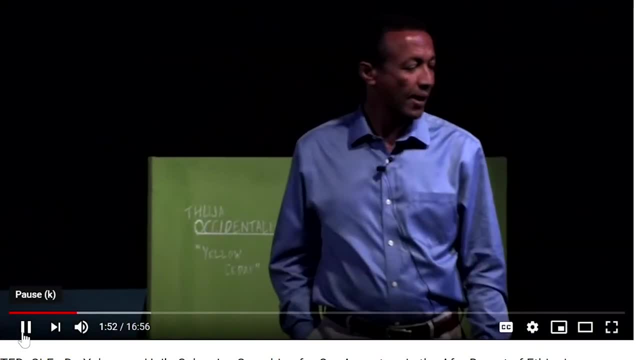 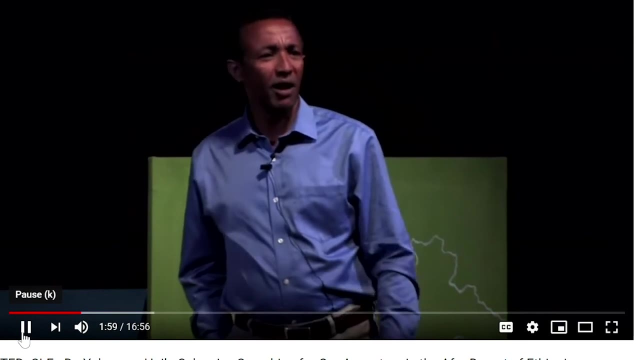 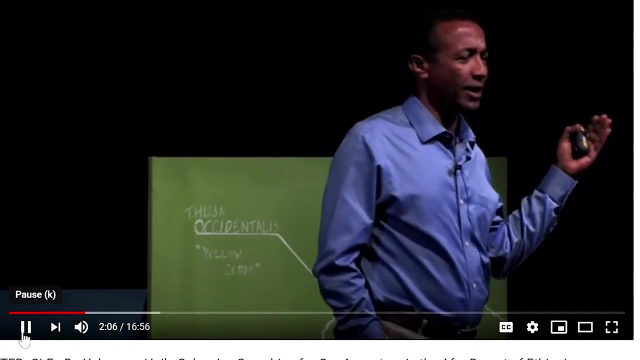 And that's why these early human ancestors used to live there as far as six million years ago. Now you might wonder: why this place? Why don't we find fossils of our early human ancestors in Ohio Valley Or why not in Death Valley in California? 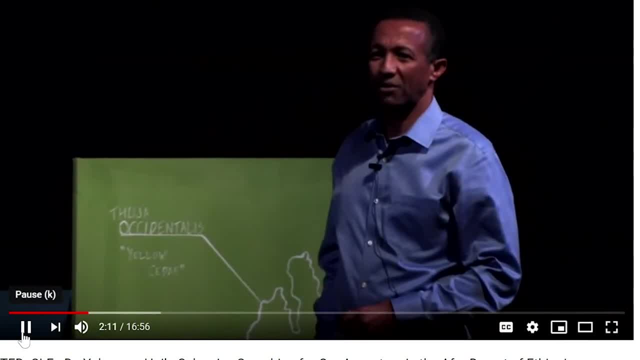 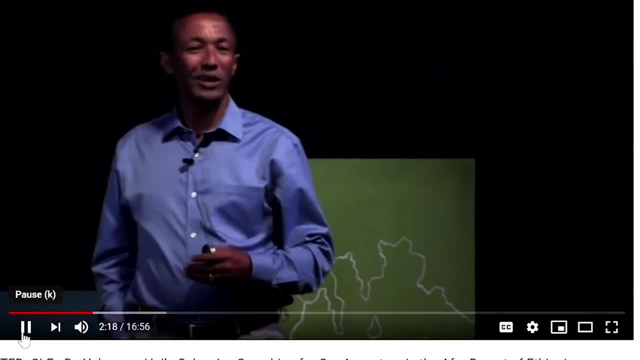 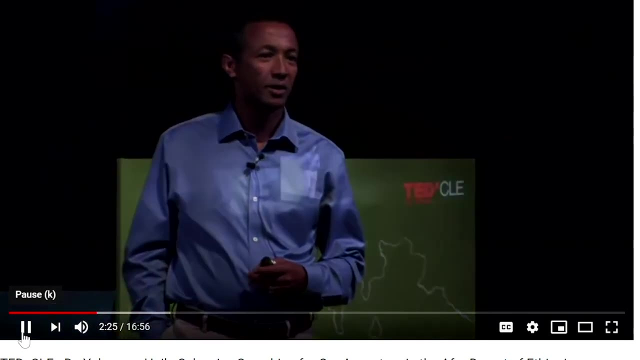 Well, unfortunately they're not there. They were never there at this time. But this place, this Afar Desert of Ethiopia, owes all its paleoanthropological fame to one geological phenomenon known as plate tectonics. Now, the Earth that we live on, 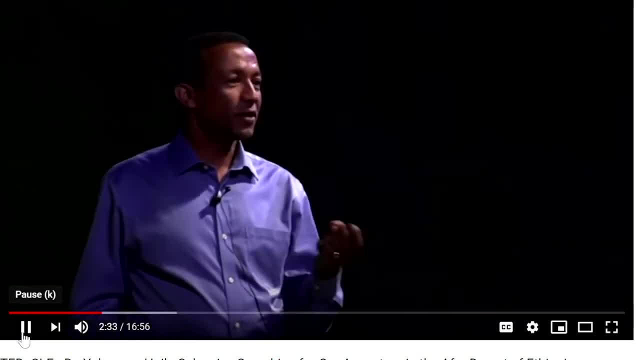 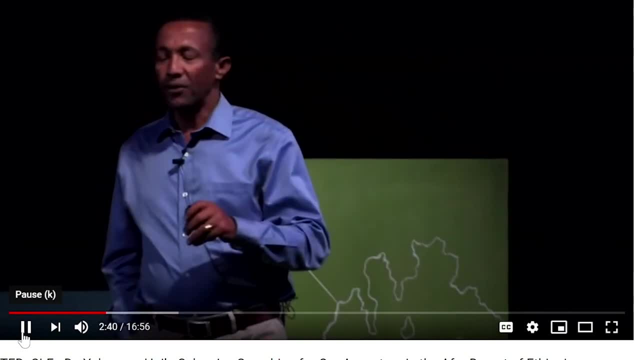 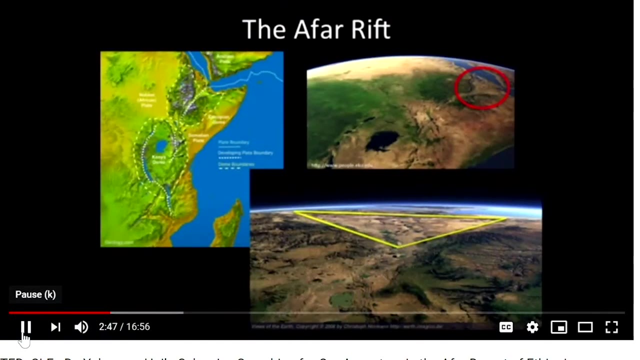 sits on what we call plates, And these plates are not still They move. They move in different directions, And there are three plates in the Eastern African region, like here, that are drifting apart from each other. Of course, some of these plates also collide. 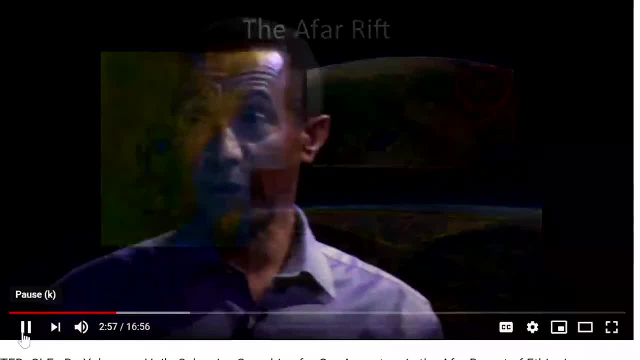 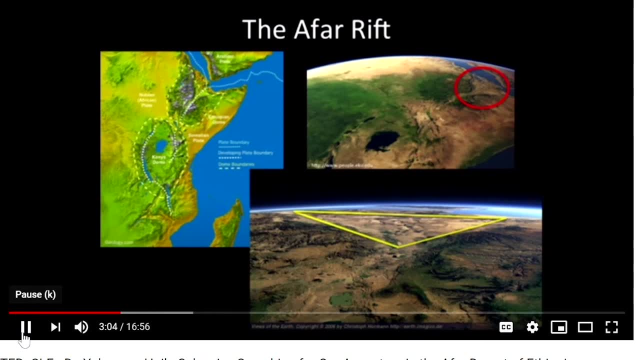 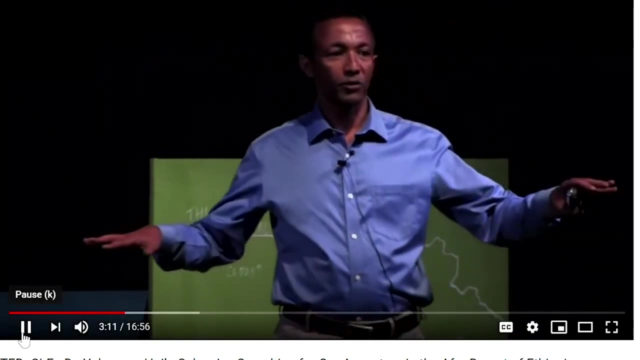 against each other and create mountains. But at this specific place, these three plates- the Ethiopian plate, the Somali plate and the Arabian plate- have been pulling apart from each other, at least for the last ten million years Now. while they pull apart from each other, 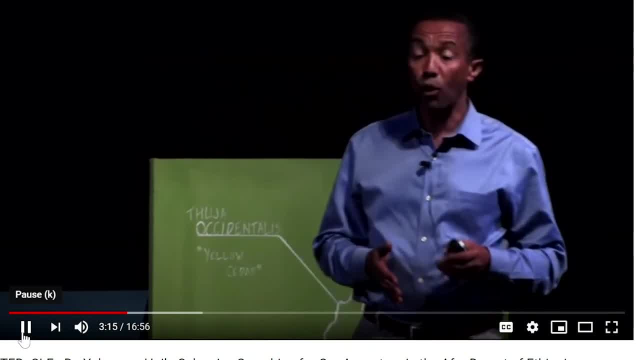 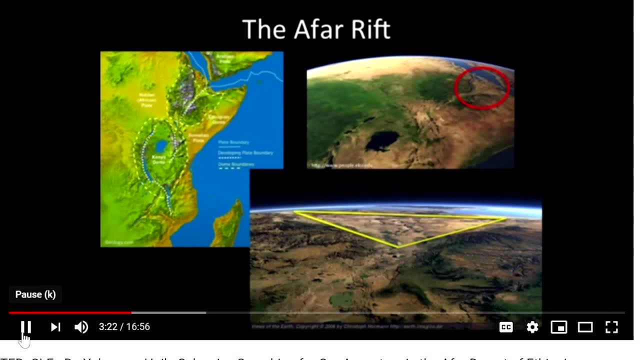 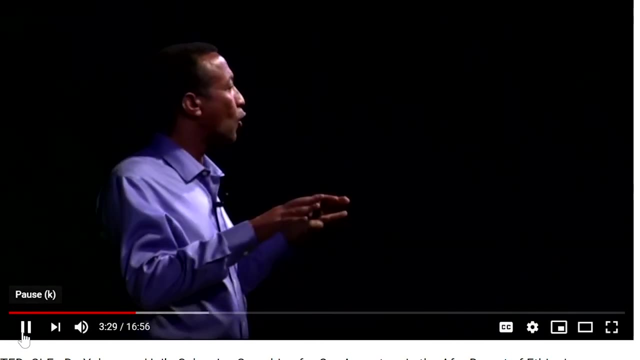 they're creating this huge crack which runs all the way from Lebanon in the north, all the way down to Mozambique. It can follow the rift all the way down to almost South Africa And while it opens, what it's doing is it's exposing these long-buried deposits. 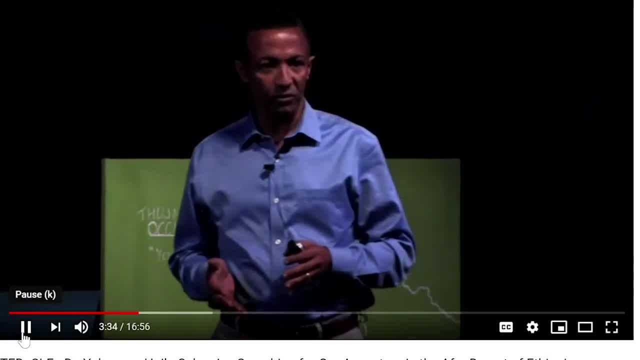 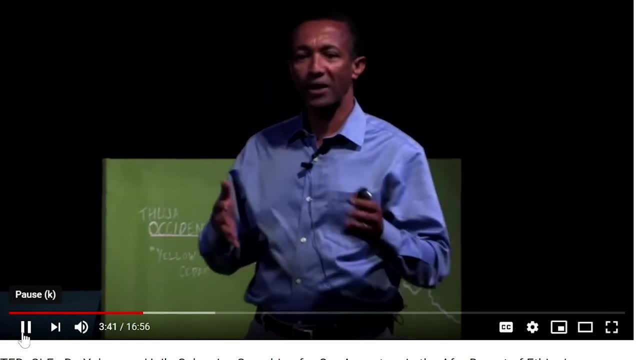 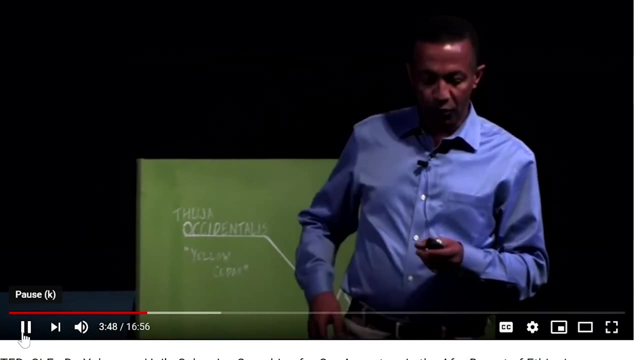 with some signature of life from millions of years ago, And erosion plays its part, exposing these signatures of past life in the form of fossils. That's what we go look for in this part of the world And, of course, what you see here on the lower part. 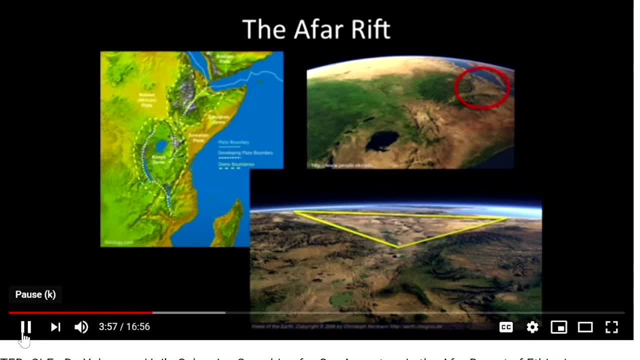 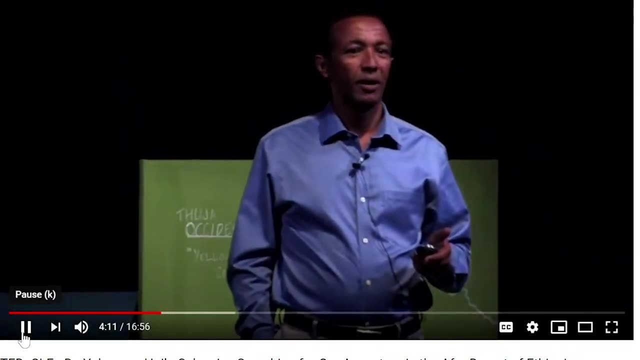 is what's called the Afar Triple Junction, because there are three different plates in this region, And this is where we go all the time. I go to Ethiopia every year, not only because I have living relatives who live there, but it happens that 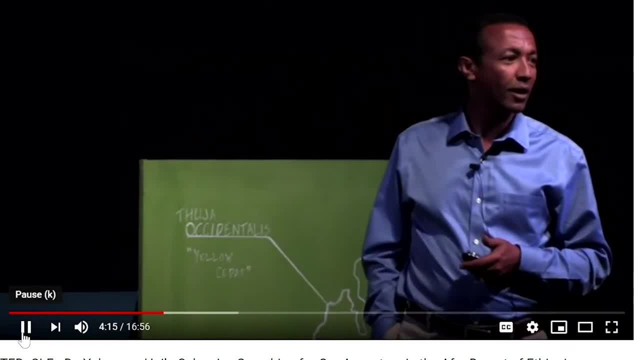 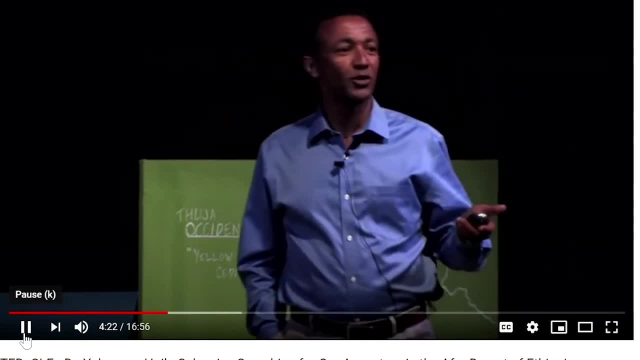 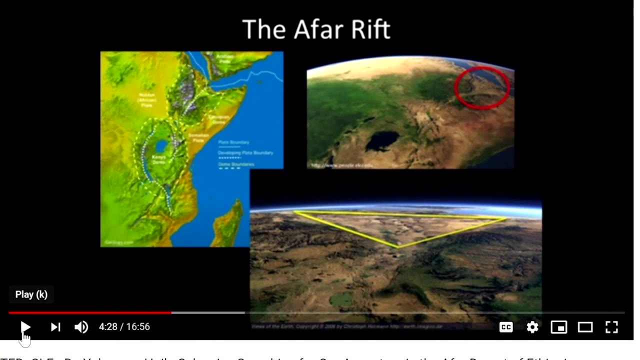 all the long-dead relatives of mine are also there. What a coincidence, Right, At least for me, Because whenever I go I happen to see both Right. So here is. So that's Yohannes Haile Selassie. 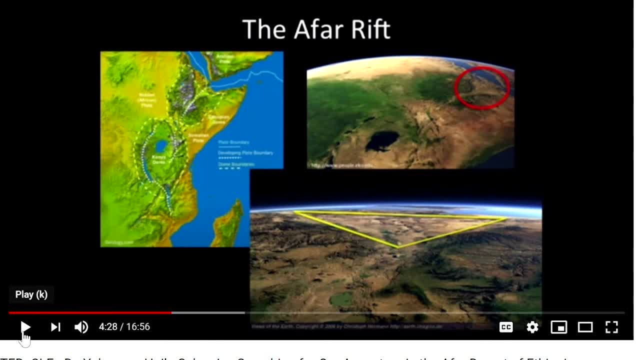 He's actually from Berkeley. He got his PhD here many years ago. And now I also want to introduce you to Dr Zarasanai Alemseged. He's a professor at the University of Chicago and used to be at the Cal Academy. 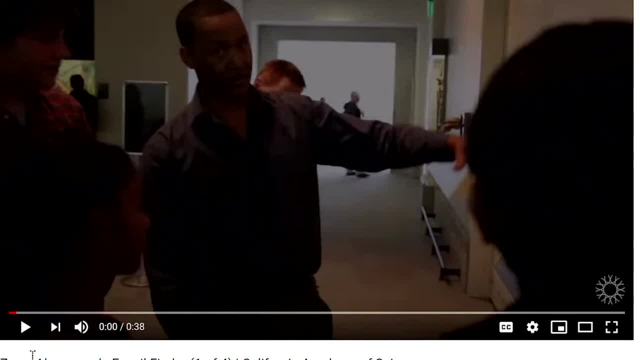 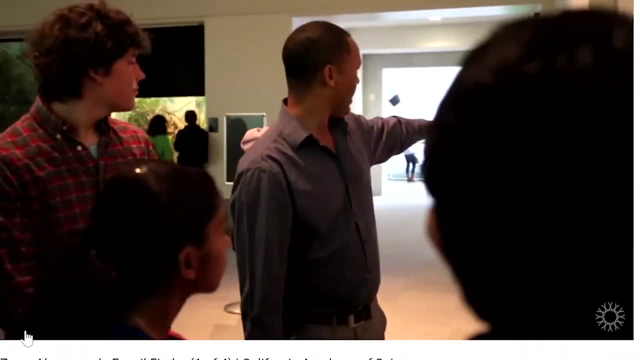 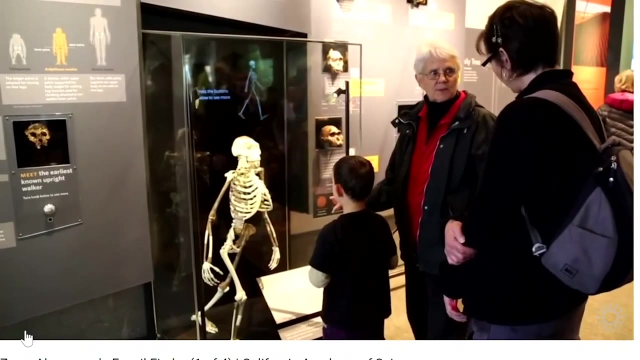 so just across the bay, And let me have him talk just for a little less than a minute. for you, Humans, by nature, are the most curious species that you can have. Therefore, when we want to understand about our past- a million, two million- 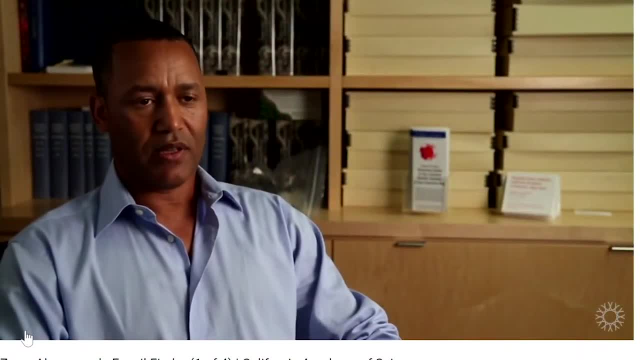 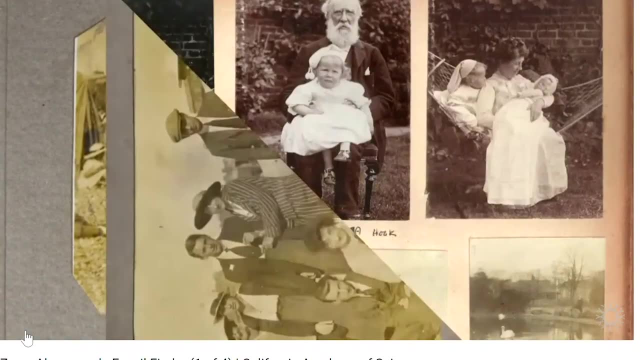 three million, four million years ago. it's nothing but an extension in time of the type of curiosity that you have to know who your mom is, who her mom is, who her mom is, etc. etc. etc. So what we do as paleoanthropologists? 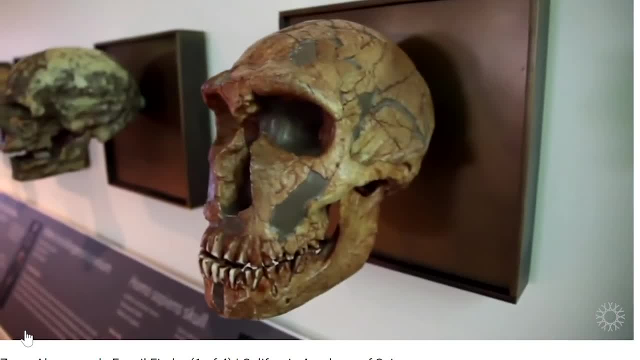 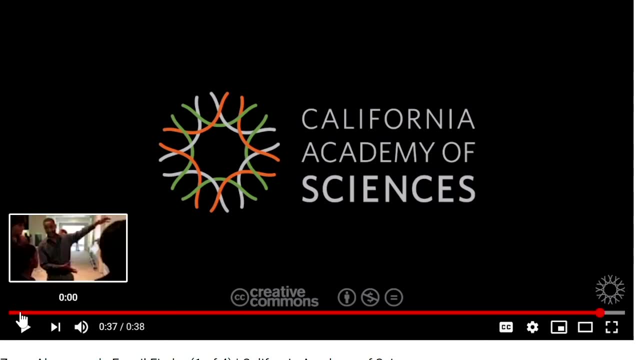 is only multiply that by hundreds and thousands of generations. Okay, so please go check them out and some of their amazing research that they've both been doing. So for now, though, let's get back to the video. I won't interrupt again. Bye-bye. 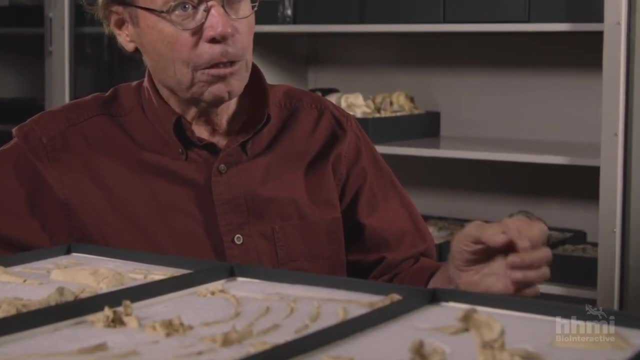 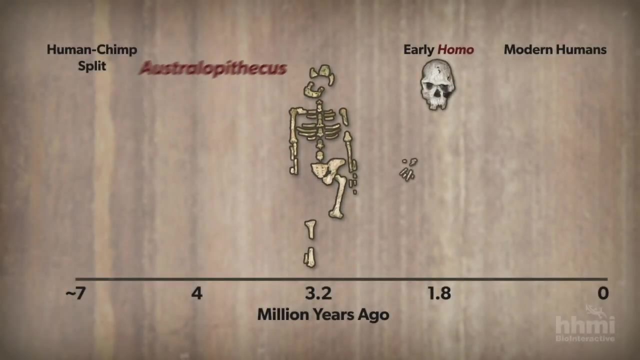 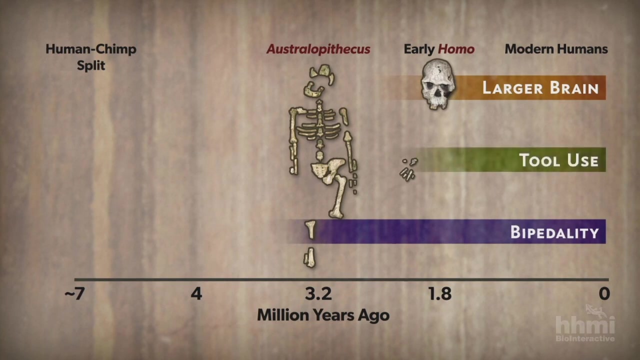 This is the Lucy skeleton found by Don Johanson in Ethiopia. She's 3.2 million years old and very representative of Australopithecus, the next earlier phase of human evolution, And they are bipeds: relatively small brains and no evidence so far. 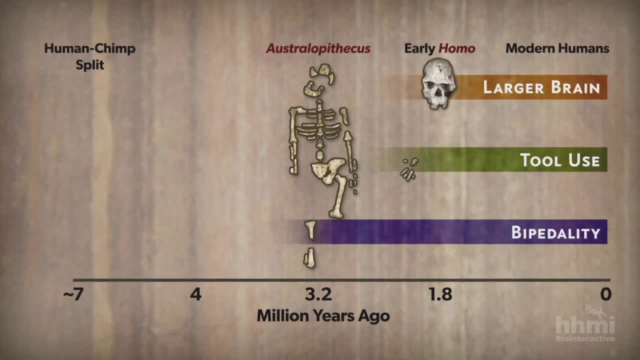 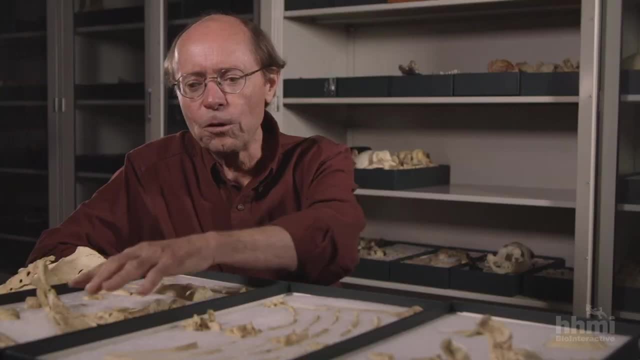 of any stone tool use. So the stone tool use comes in much later than Lucy and her brethren, With early Homo. What do we know about this creature from the fossils? When we look down here into the pelvis, we see evidence for bipedal walking. 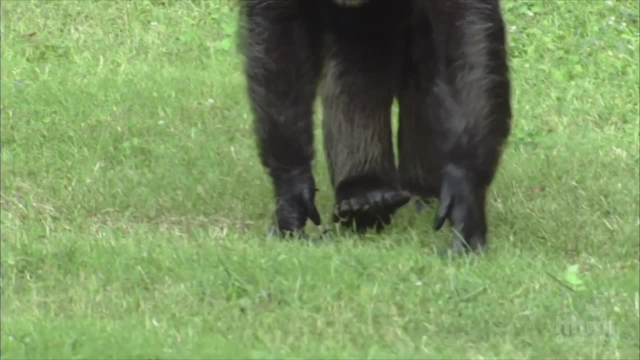 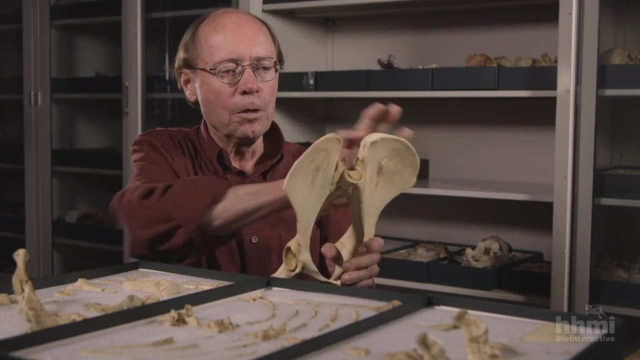 a commitment to walking on two legs. that is very different from what we see among great apes. So when we look at a chimpanzee in the hip, we see the hip bones behind. They're long, they're tall, they're up the creature's back. 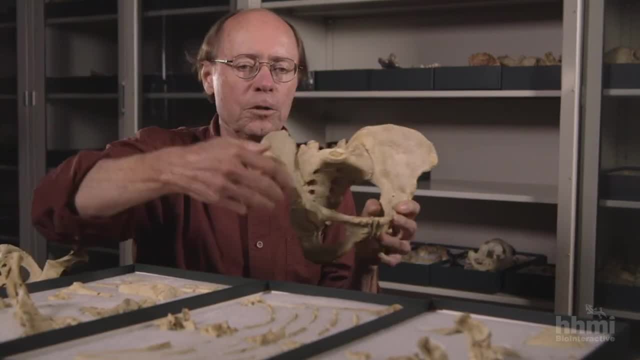 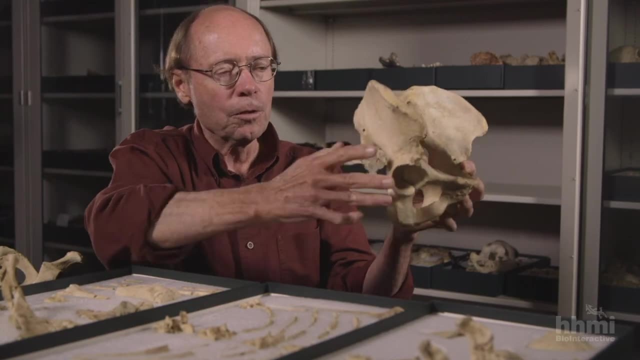 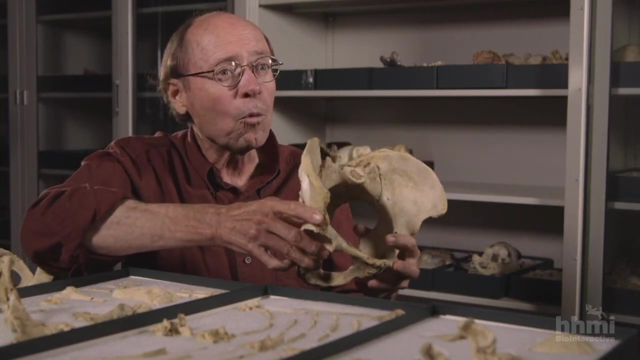 Whereas in a human our hip bone is much broader, front to back shorter and wrapping around the side to put these muscles that control pelvic tilt during walking in an advantageous position. Then we can ask the question: is Lucy more like a human or more like a chimp? 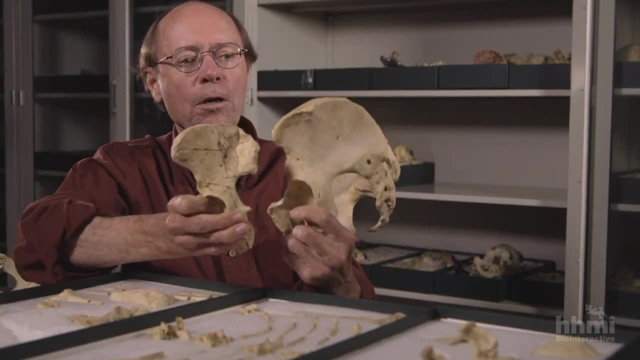 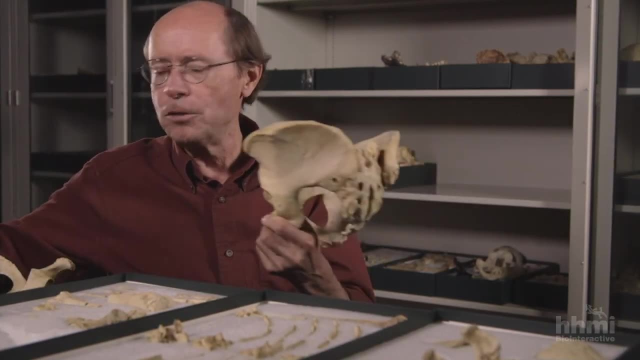 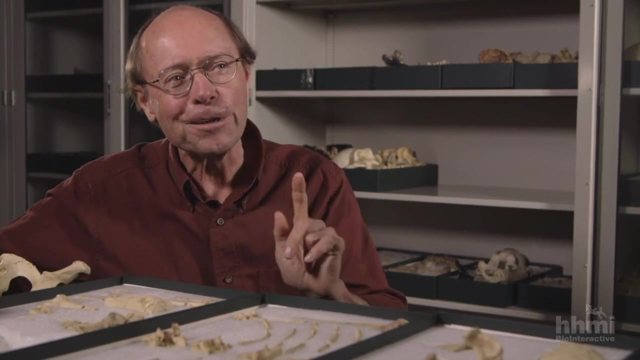 She has a very short blade on the pelvis, much more like a human. She has muscle attachments, much more like a human. It's a basically bipeds architecture And that's how we know she's a human. But there was a little bit of controversy. 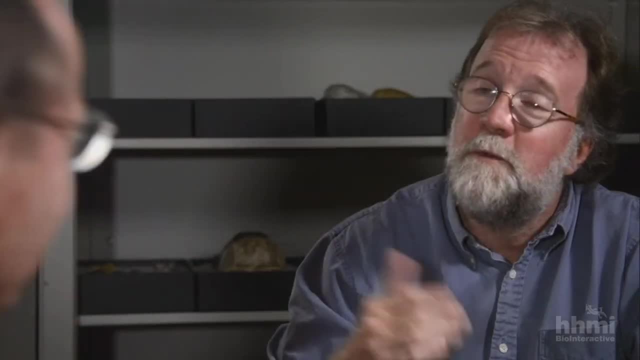 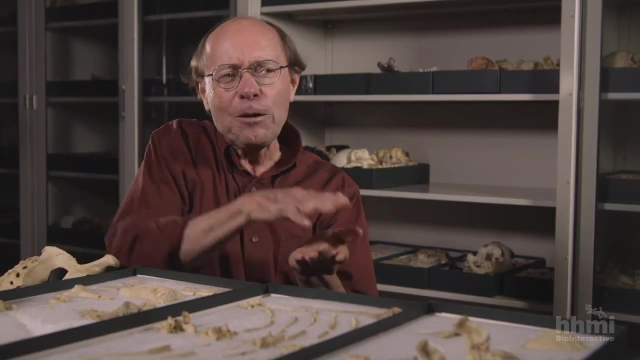 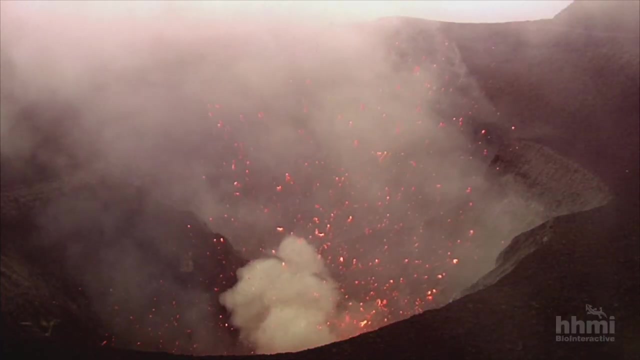 Even after that, some people said: well, how can we really be sure about that? And how can we be sure? Because we found these incredible things in northern Tanzania, older than Lucy, sandwiched between layers of volcanic ash, And it's not what you think. 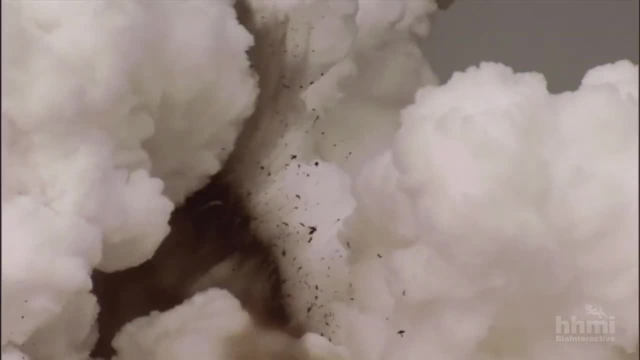 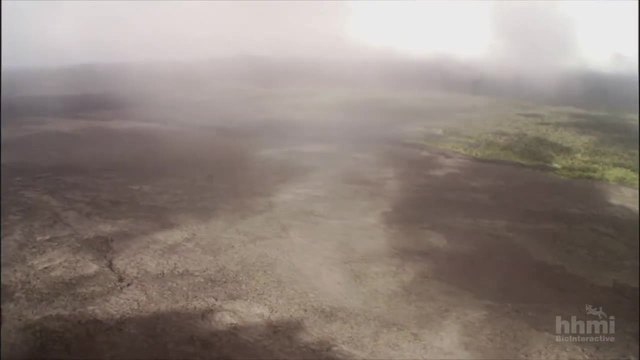 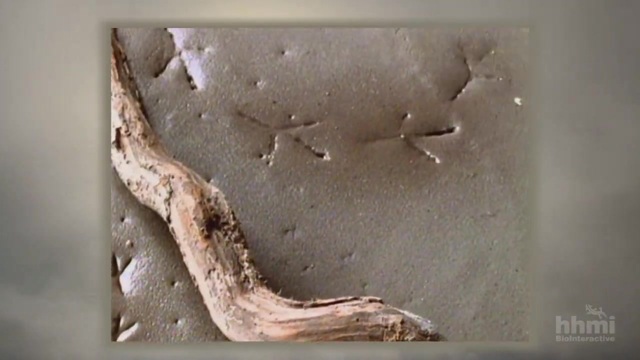 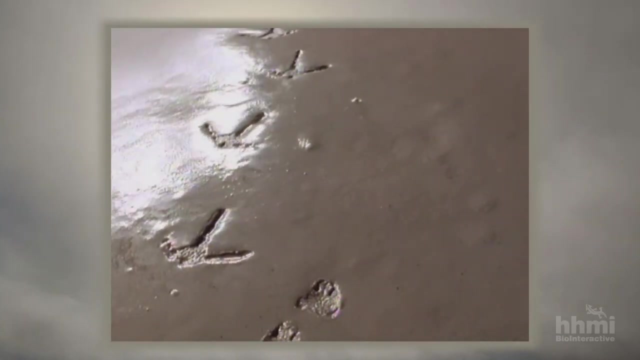 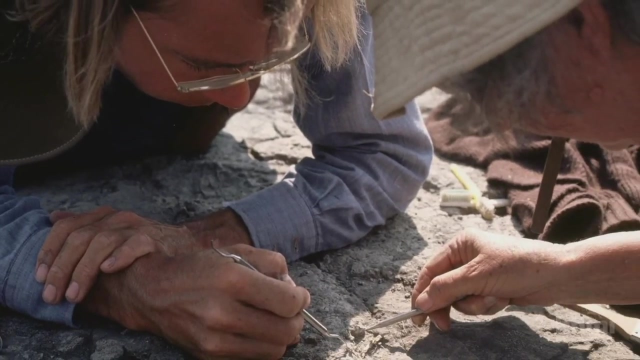 It's not bones. There was a volcanic eruption 3.75 million years ago. The volcanic ash came down on the Serengeti Plain And animals walked across it. The ash hardened and was buried In the 1970s. 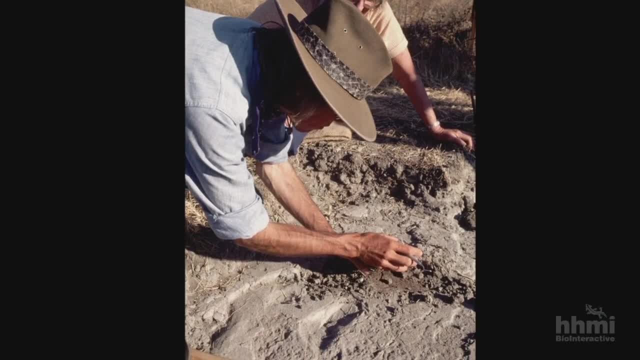 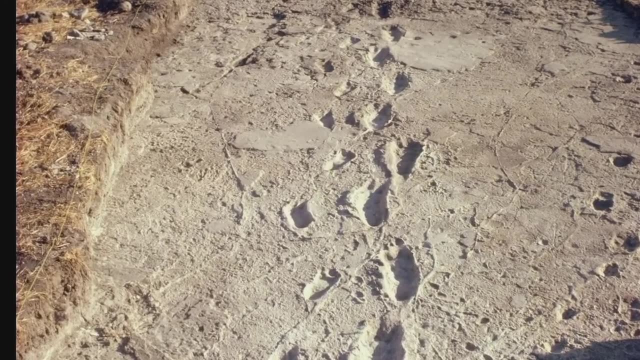 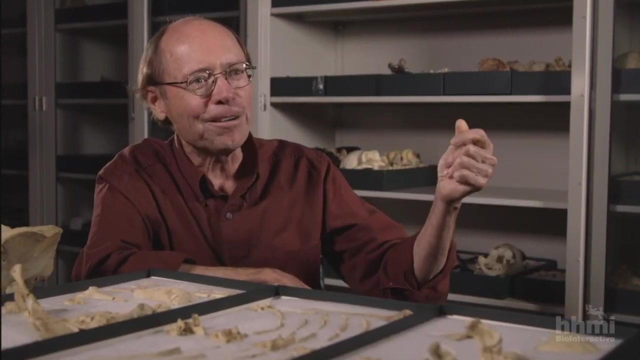 I was lucky enough to be with Mary Leakey out in this area and we found the trails of hominid individuals left as they walked across that volcanic ash millions of years ago. It was an amazing, like a snapshot of time. They went for meters. 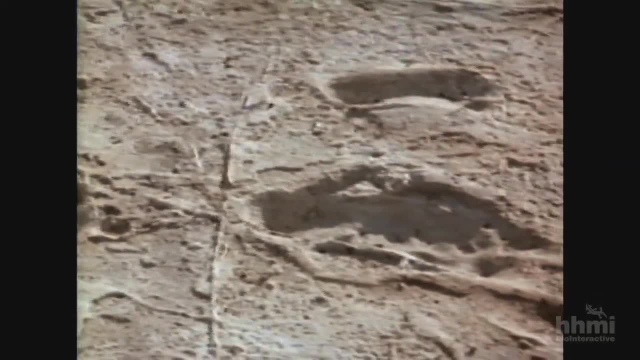 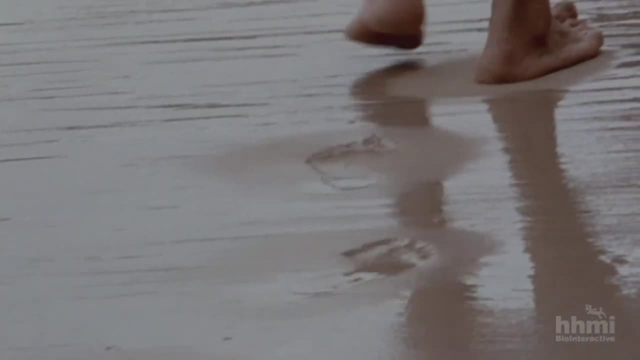 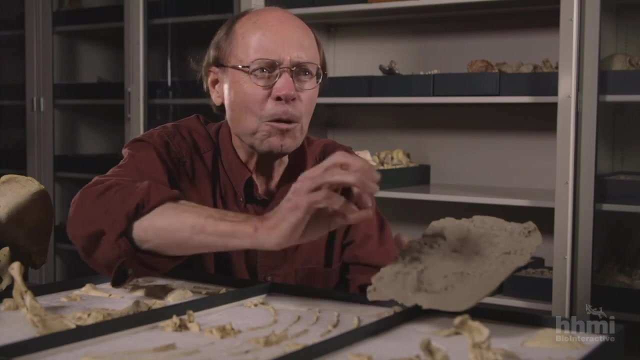 and meters, and meters. There are no knuckle marks, no handprints, just bipedal footprints. It looked more or less like what a guy would leave on a beach. Human feet- we're all used to them, but they're really strange. 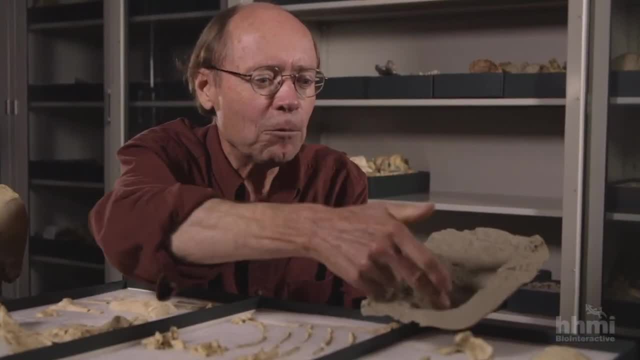 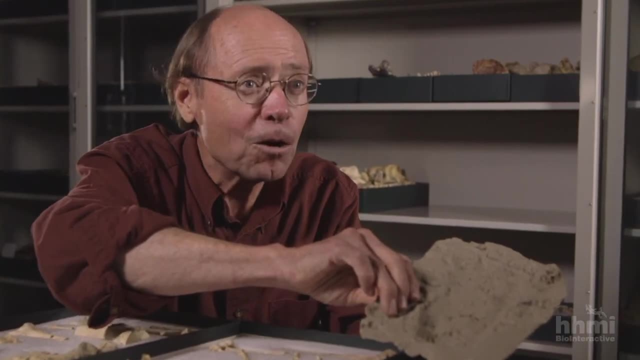 Our big toe is in line with our other toes. We don't have a grasping big toe. We have arches, transverse and longitudinal in our feet. All these features are present 3.75 million years ago in Australopithecus. 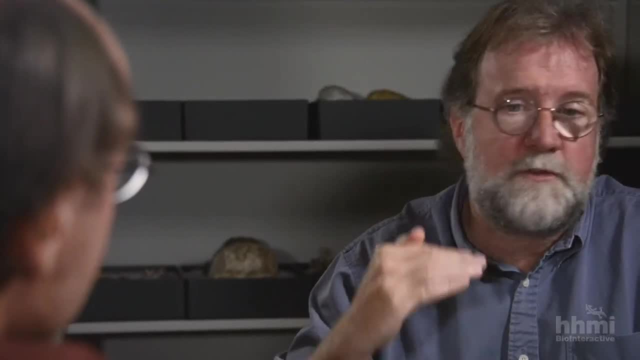 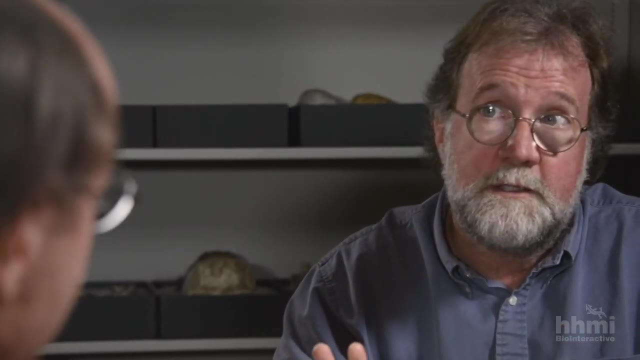 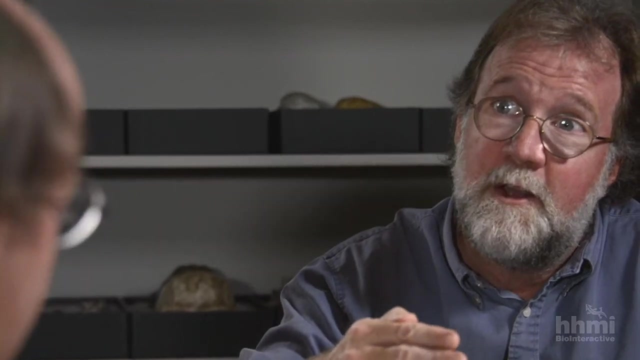 So Australopithecus pushes us all the way back to 3.7 million years or older. She's small brained, not using tools to our knowledge, but walking upright. So that's telling us that walking upright is yet still an earlier trait. 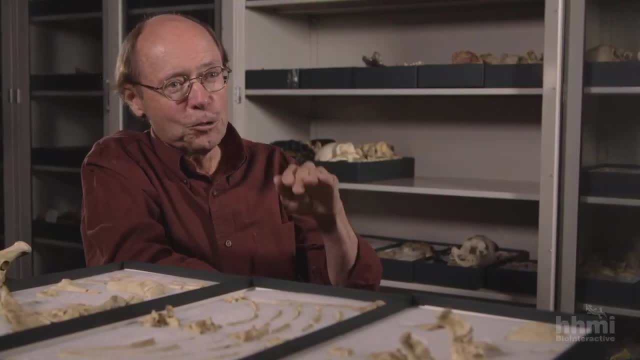 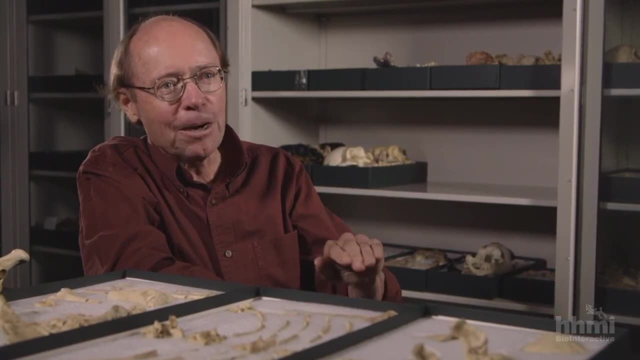 What do we know about that? We didn't know very much about it because Lucy and her species only went back to 3.75.. So to take the next step back in time, we had to find older fossils Just 50 miles south. 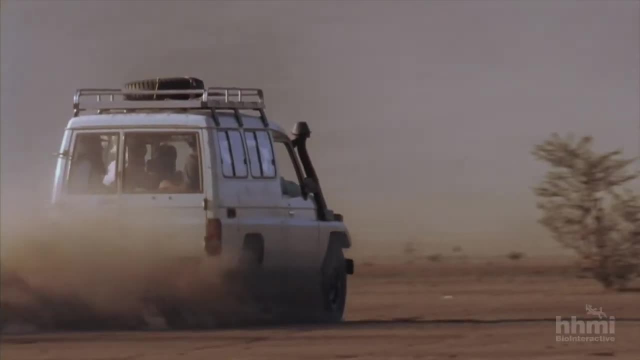 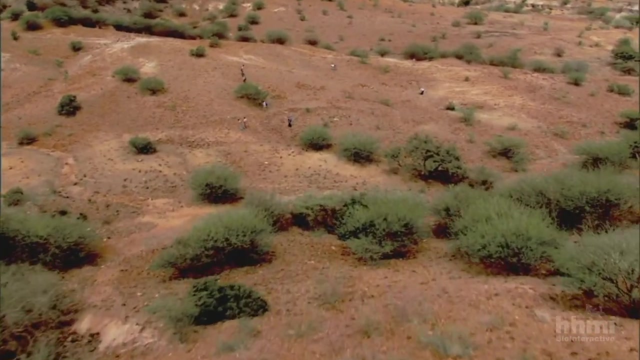 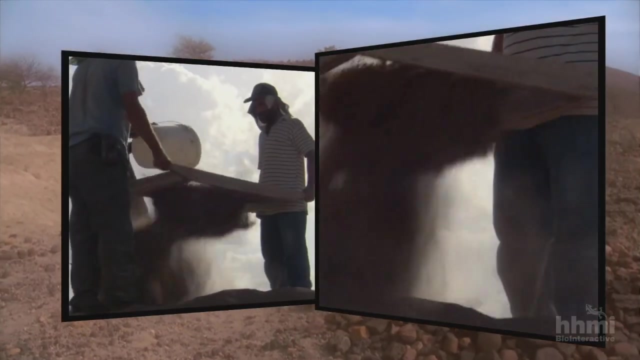 of where Lucy was found, there are exposed rock layers reaching back 6 million years. This is where Tim White and a large international team of geologists, paleontologists and archaeologists have focused their combined efforts since the early 1980s. 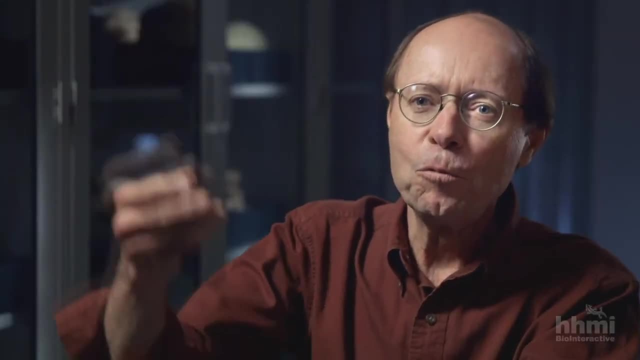 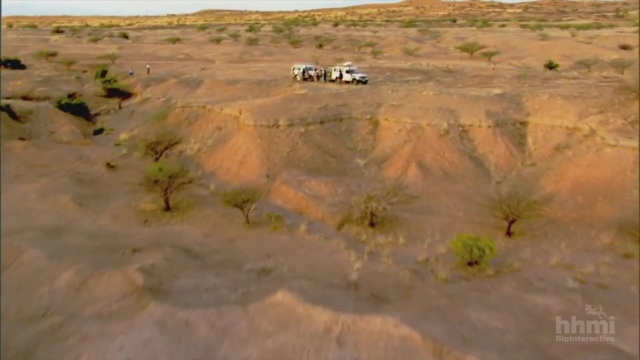 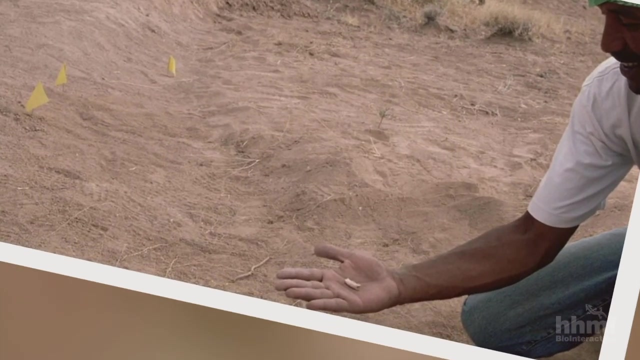 What we wanted to do was to plumb the unknown, to figure out what came before the Lucy fossils. For a decade, what they'd come for largely eluded them, until A graduate student at the time, Johannes Haile Selassie. 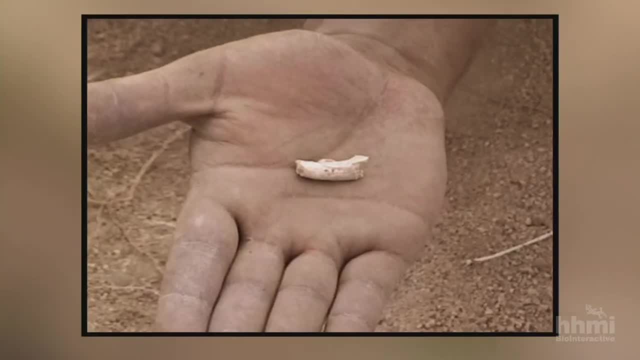 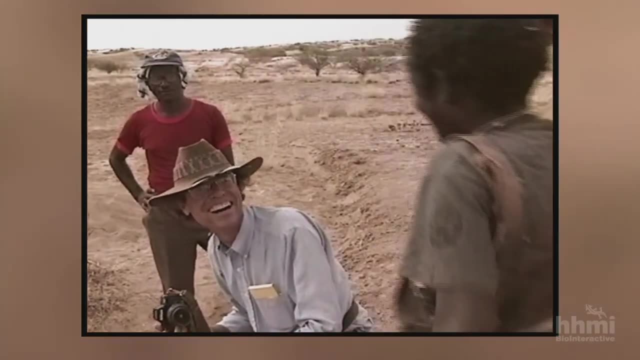 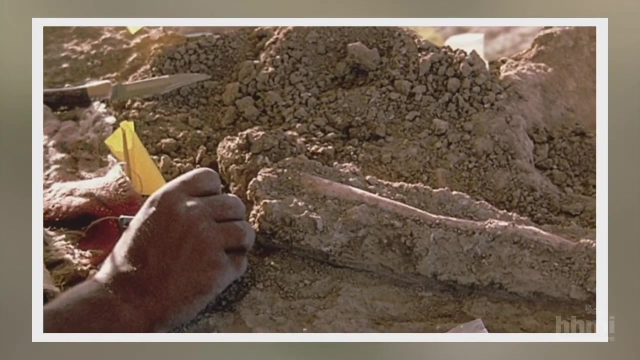 found two little pieces from the palm of the hand. just this bone here and these little pieces. he picked up and said: this looks like a hominid. The excitement of this and other early finds made it possible for us to find more of these. 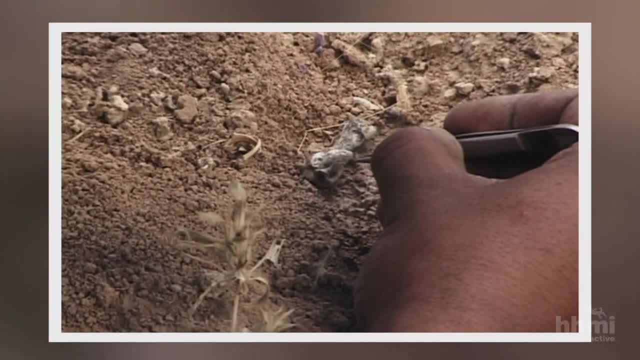 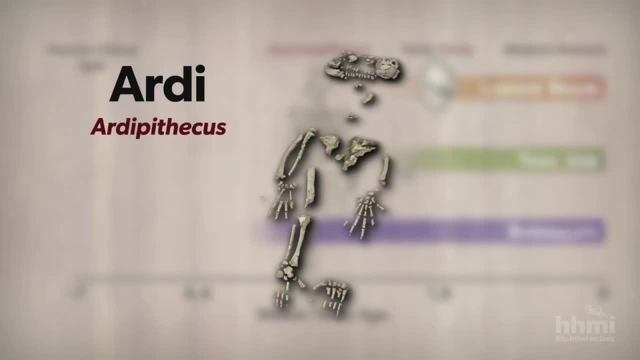 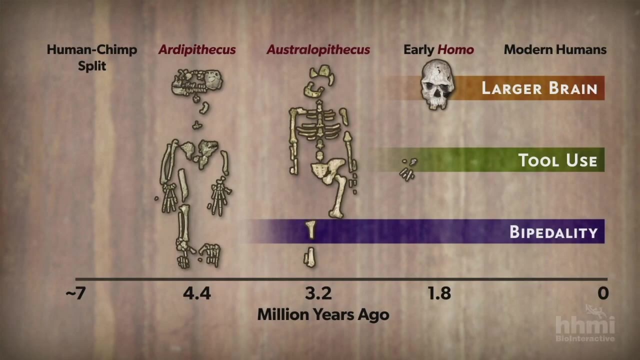 Hand, foot, arm, leg, teeth, skull, head to toe. we had coverage of a creature nobody had ever seen before. We nicknamed her Ardi for the genus Ardipithecus. The species is Ramidus and it's really a skeleton. 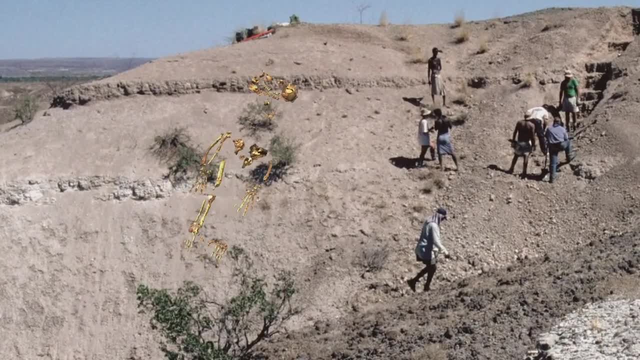 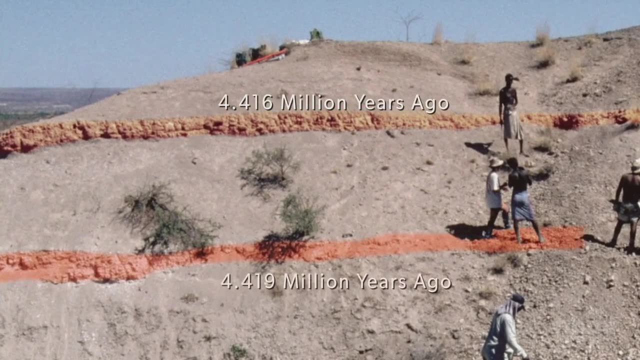 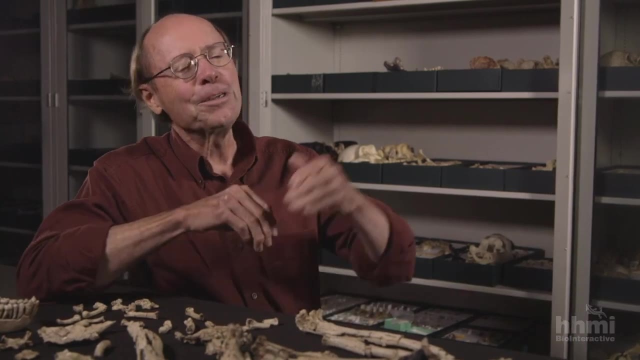 that is representative of the earliest known phase of human evolution. They were all found sandwiched between volcanic horizons, both dated to 4.4 million years ago, So that's more than a million years older than Lucy. It was stepping into that. 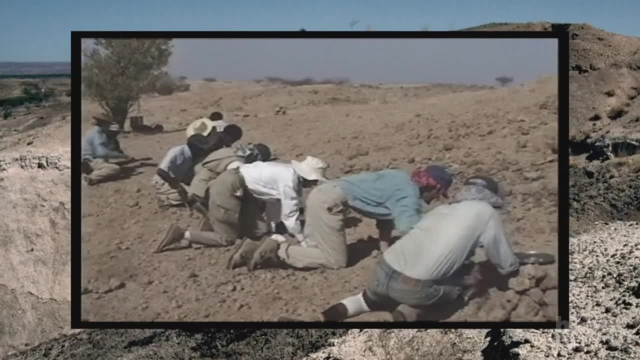 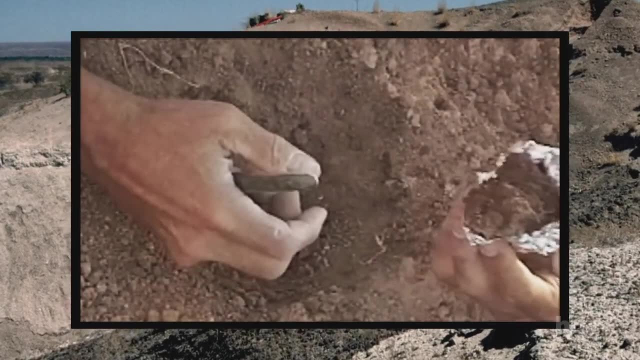 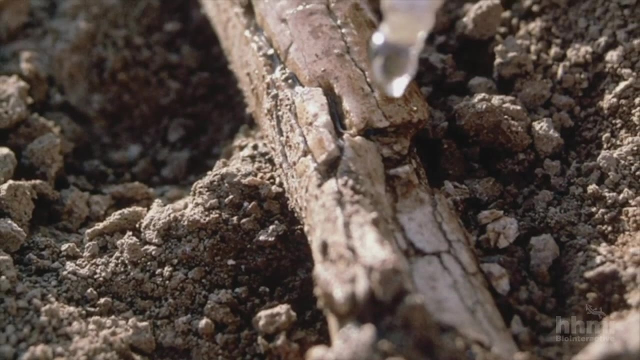 black hole beyond Lucy that nobody had been able to step into before Removing Ardi from her 4 million year resting place was a real challenge. Her bones were ready to turn to dust. They had to use chemical hardeners on her extract her in plaster jackets. 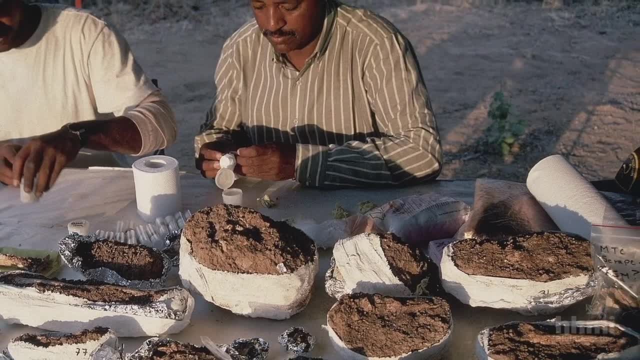 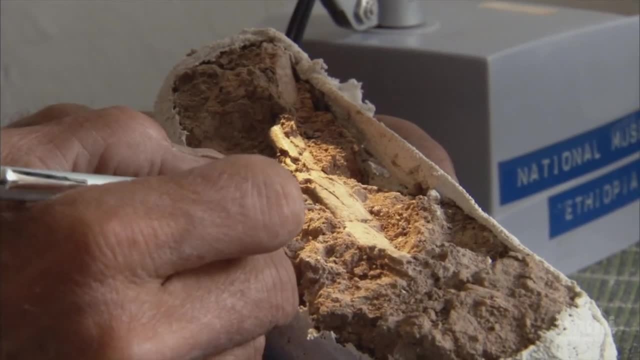 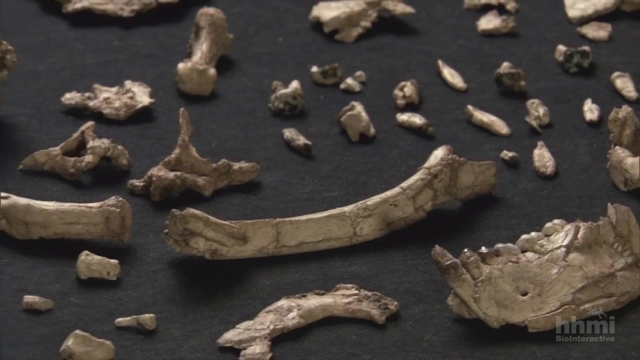 and then work on each bone under a binocular microscope with a needle to clean the encasing sediment from the soft bone underneath. But what we got as a result of that is a really unrivaled look at the anatomy of a very ancient hominid. 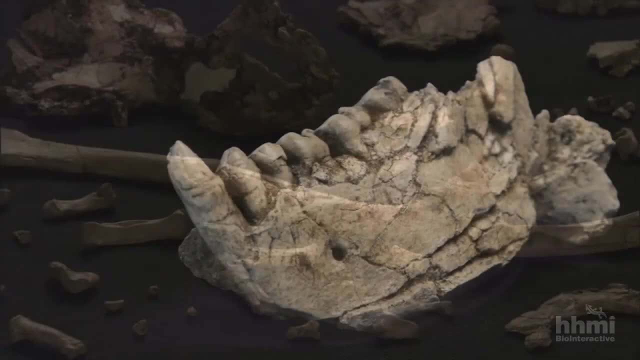 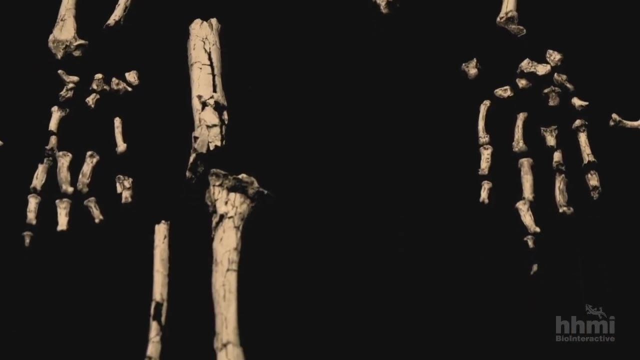 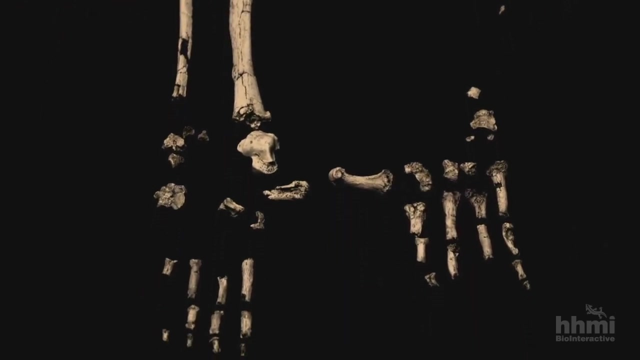 We could see the muscle attachments on the finger bones. We could see the scratches on the teeth. It's beautiful anatomy With some real surprises. especially below the neck, There was an extension in the lower pelvis that showed that she was a climber. 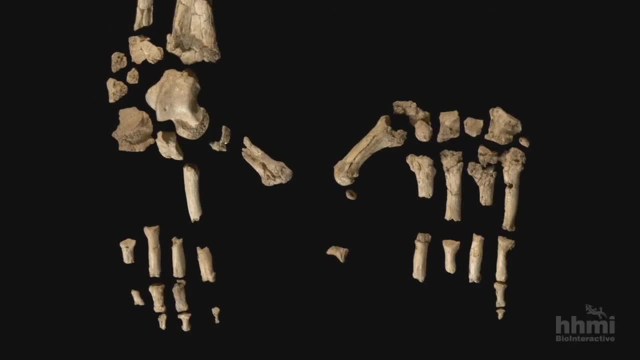 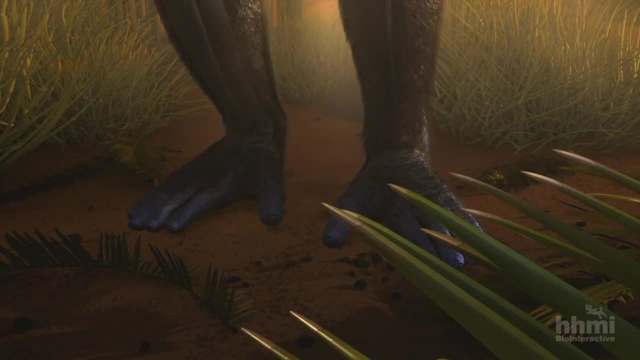 In the foot, a large toe that stuck out to the side of the foot. the first time this is ever seen in a hominid, even though all other primates have this. She is this peculiar mosaic with bipedality on the ground. 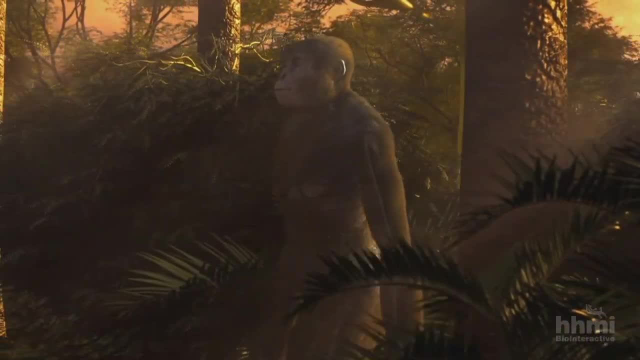 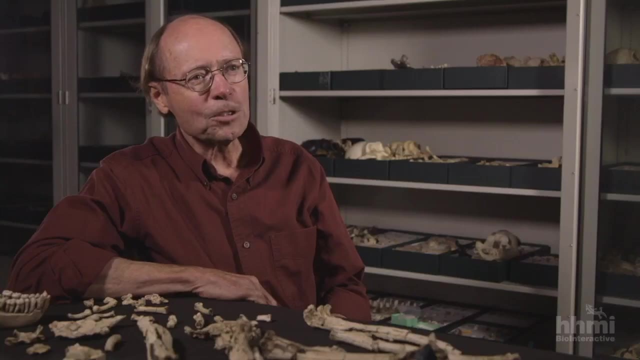 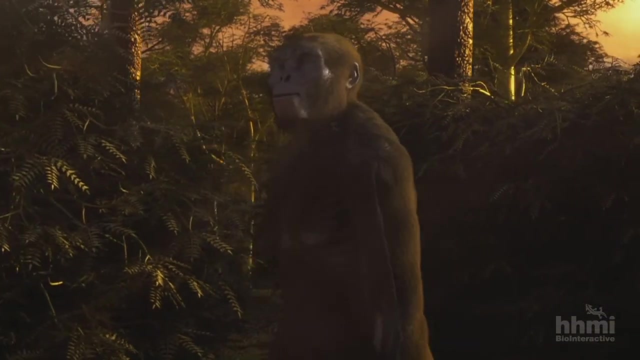 but also climbing abilities far superior to those seen in later Australopithecus. You couldn't possibly have expected this. Nobody could have expected it, because you can't predict this from looking at chimps and humans and triangulating. Artie is neither a chimp. 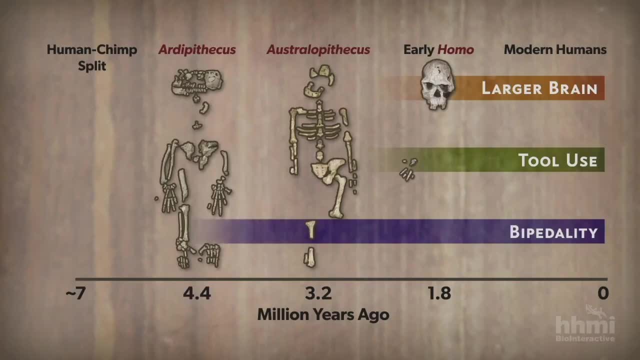 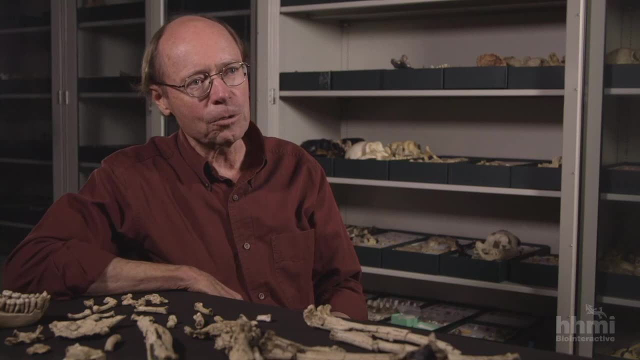 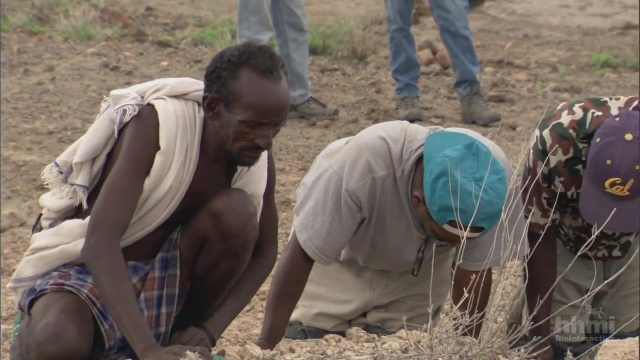 nor is she a human. She is a mosaic, 4.4 million years old, The step beyond Australopithecus. the glimpse into that first phase of hominid evolution, Buried along with Artie, was fossil evidence of the habitat in which she lived. 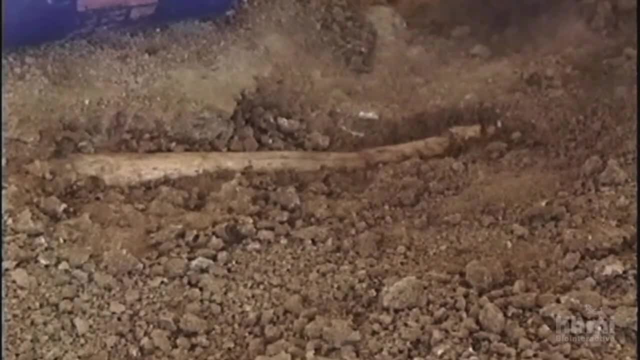 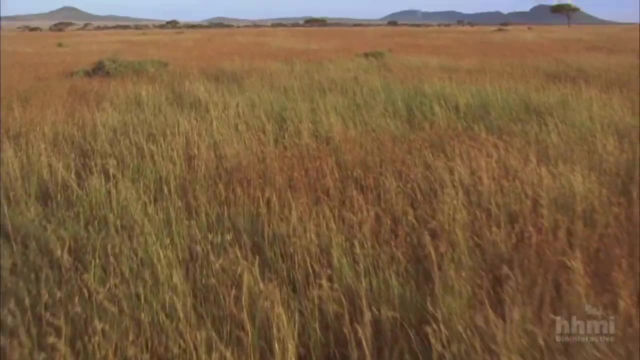 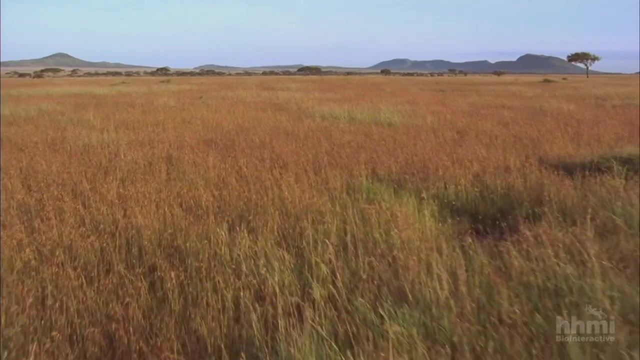 and where bipedality evolved. It wasn't what anyone had been expecting. For a long time, scientists predicted that bipedality had evolved in a grassland. The savanna has always played a big role in people's speculation, And what we had with Artie- 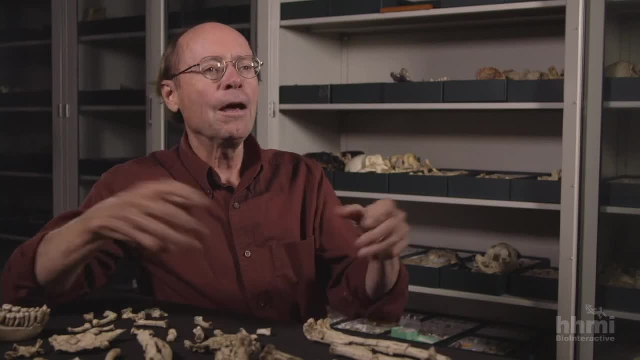 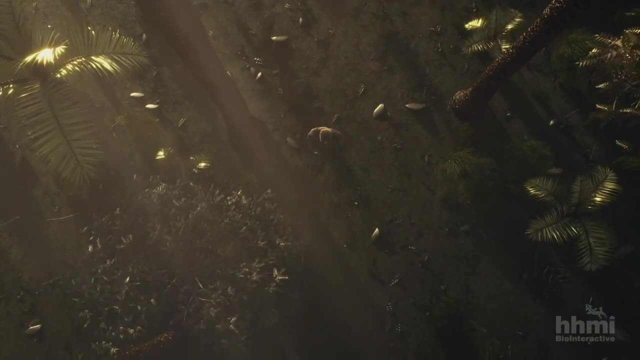 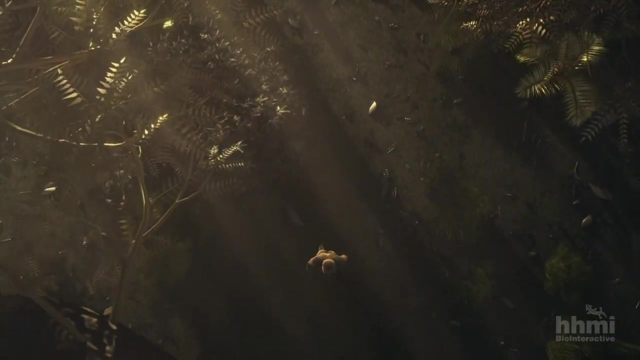 was evidence from her body and indeed her chemistry, as well as evidence from her environment, that showed she was not adapted to an open grassland savanna existence, even though she had already achieved bipedality. That evidence included tens of thousands of animal and plant fossils, indicating 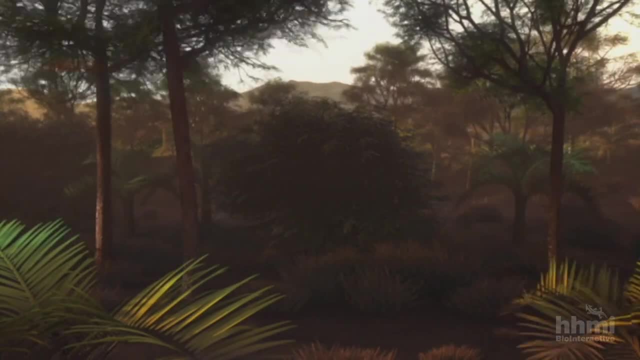 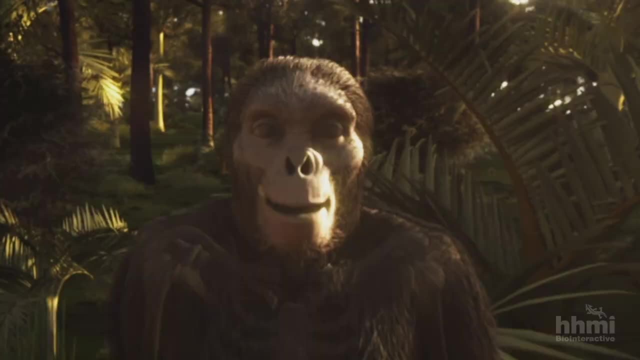 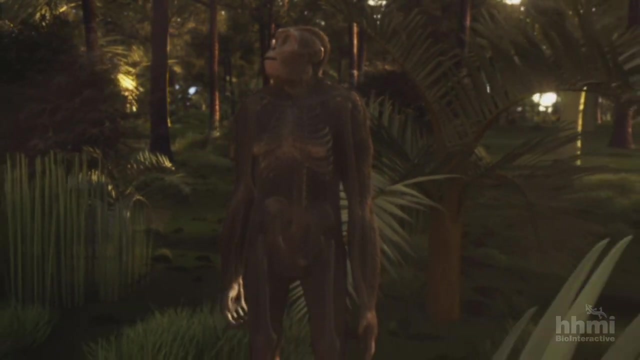 that she was living in a woodland setting, not an open African savanna. So bipedality evolved while our ancient ancestors were still spending time in the trees. Artie Pythagoras took away any doubt that bipedality was ancient And it was so ancient. 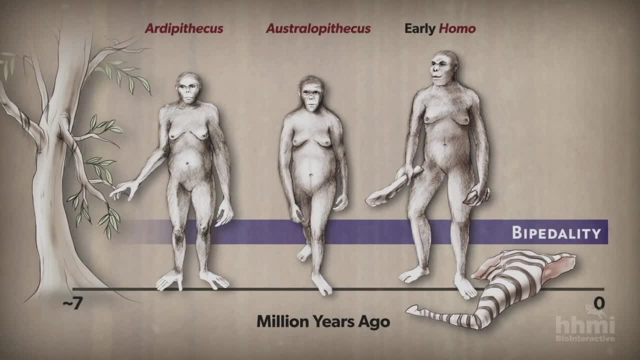 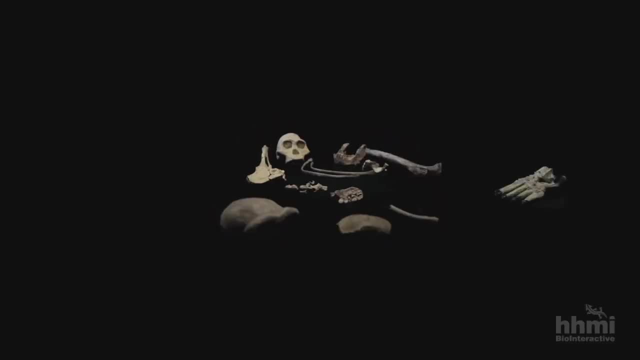 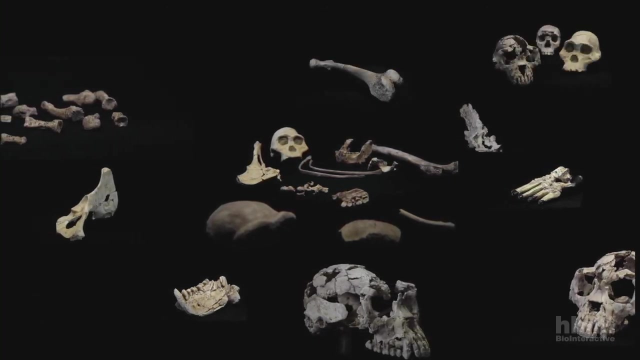 that it preceded by over a million years the expansion of the brain, the incorporation of stone tool technology. We now have thousands of hominid fossils from the past six million years. They reveal several phases in the biological evolution of humans. You have an early phase. 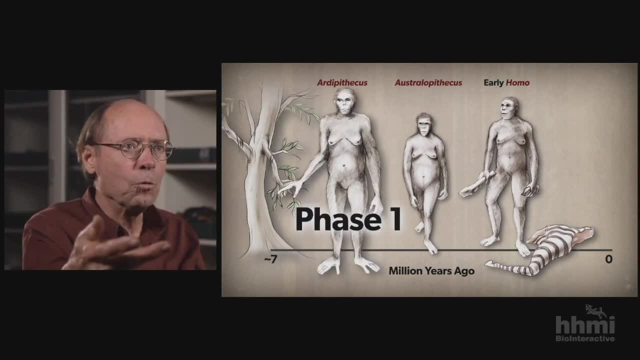 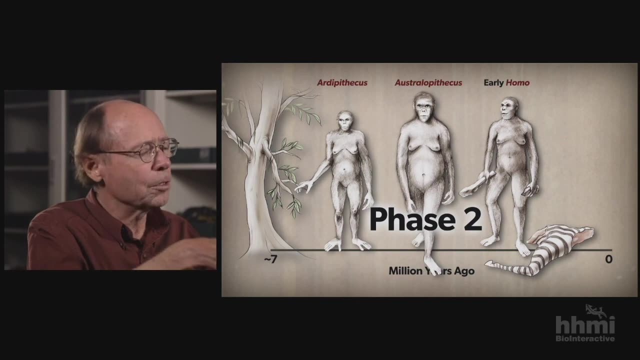 Artie Pythagoras, whose anatomy allows it to climb in the woodlands and walk on two legs. We see Australopithecus as the next phase, Lucy, a representative of this. They have real big teeth for chewing, big, robust faces. 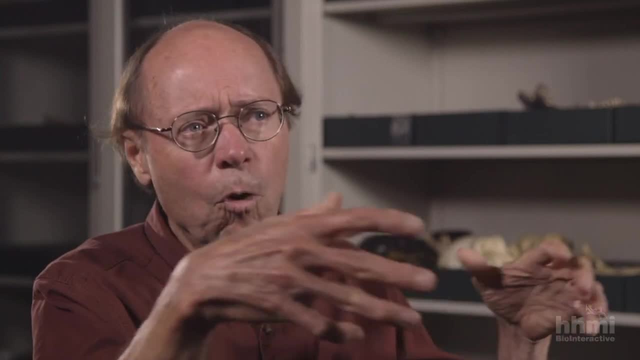 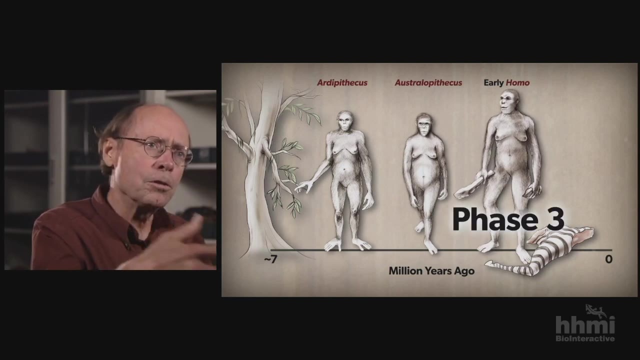 Their niche has expanded beyond Artie Pythagoras. They're in more open habitats, They're found throughout the African continent. And then the third phase of human evolution is our own genus, the genus Homo, And here we have a creature that really is a technological 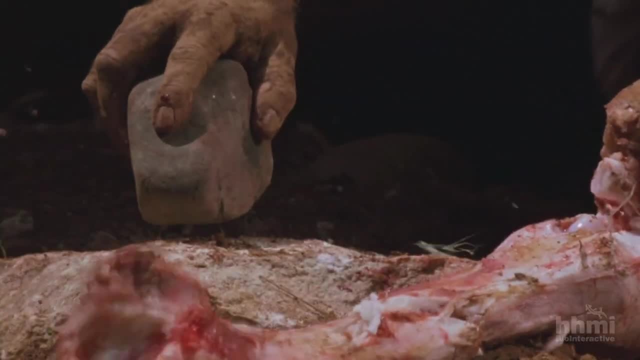 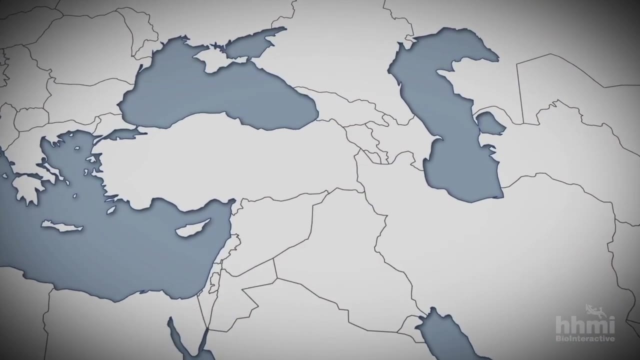 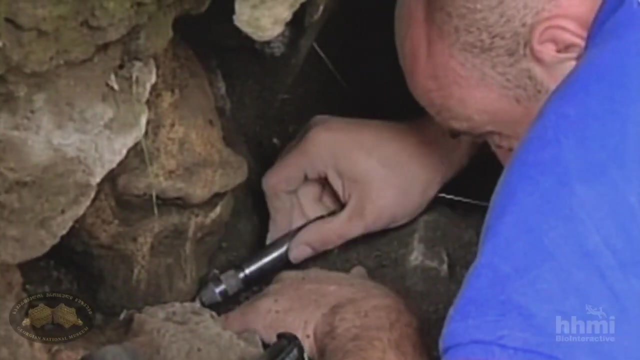 primate. depending more on the species, They broaden their diets and ultimately, their geographic range, leaving Africa. Recently in the Republic of Georgia, hominid fossils were discovered that are as old as the Olduvai fossils. They include the most complete. 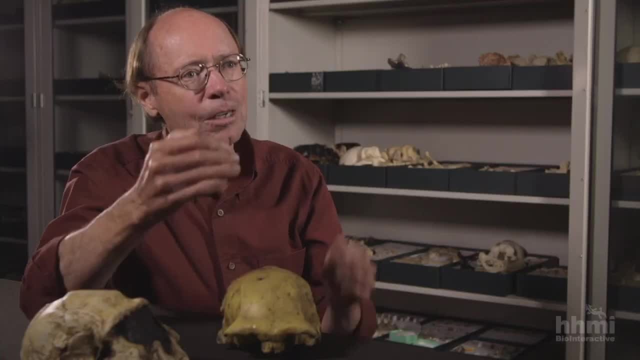 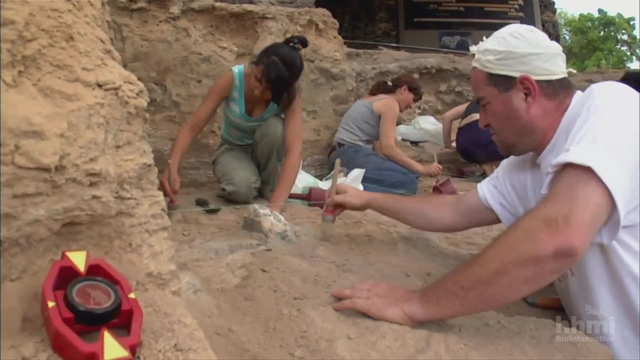 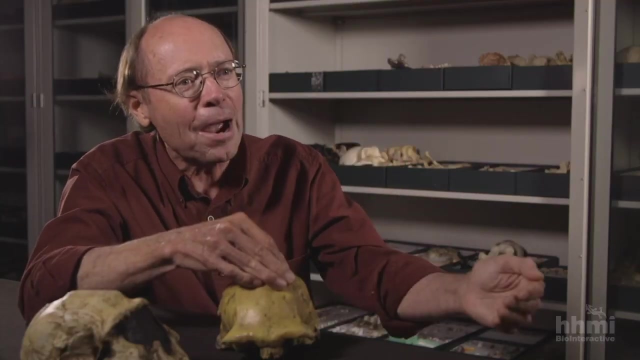 early Homo skull ever found. That is going to give us insight into the biology of our ancestors, the ancestors of Homo sapiens. This is a demonstration of how paleontology is not a dead science. Paleontology is the science by which we learn about our past.